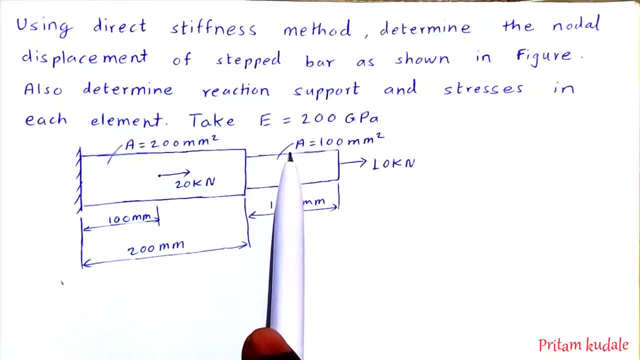 So whenever there is a change in cross-section area, there should be a node, Means it will have a two different element at left side as well as right side. So here we have to generate one node. Now again, there is one more rule: that if you want to apply any load, you can only apply it to the node only. 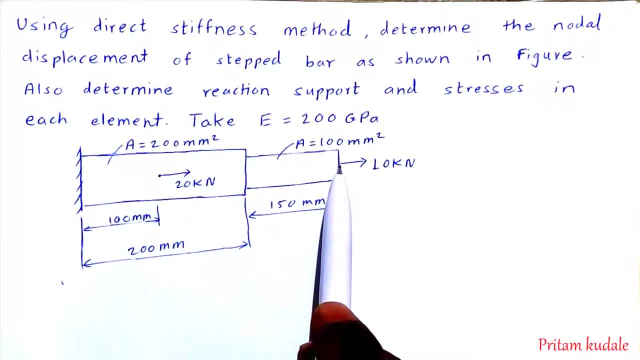 So At this particular position, this is the end of the element. so there will be a node In this particular position if you want to apply the load of 20 kN. so even this is the same cross-section. we cannot consider it as a single element because 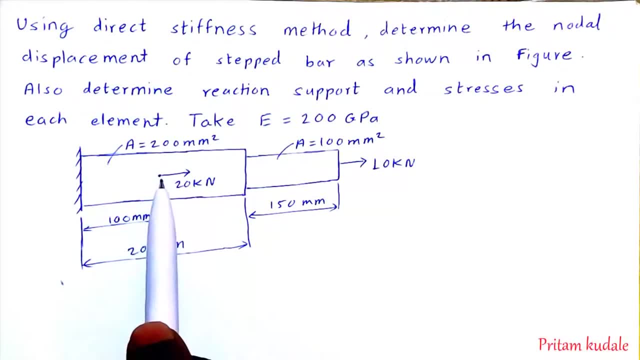 we want to apply the load of 20 kN at the mid position. So here also we have to take a node. So if we want to take a node and we are going to consider the two-noded 1D element, we have to create a separate element. 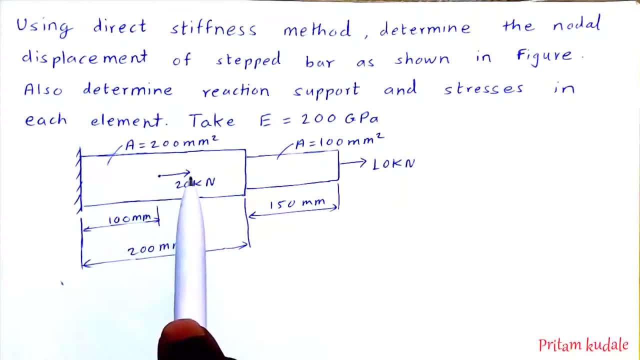 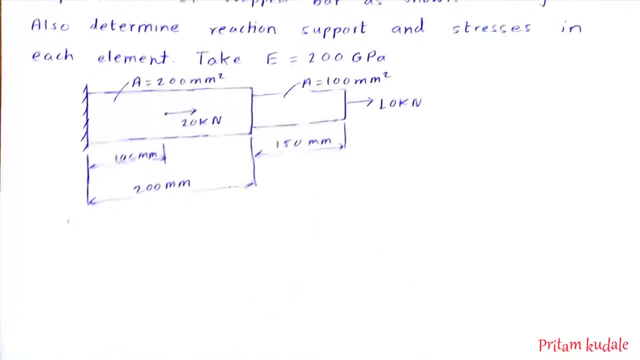 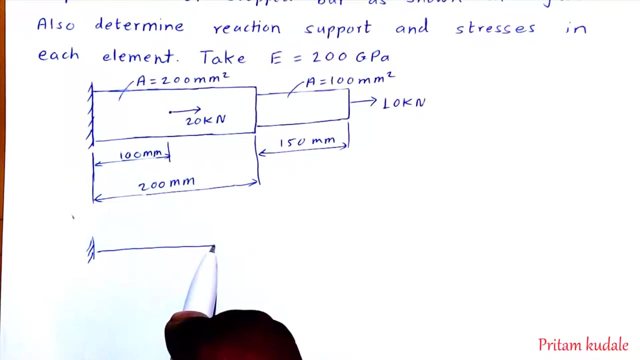 element on left side of the node and right side of the node. So we are going to divide this particular problem into the three nodes, So it's equivalent representation. we can draw it as a 1D element, So you have to draw equivalent line. then this will be your pick. support will. 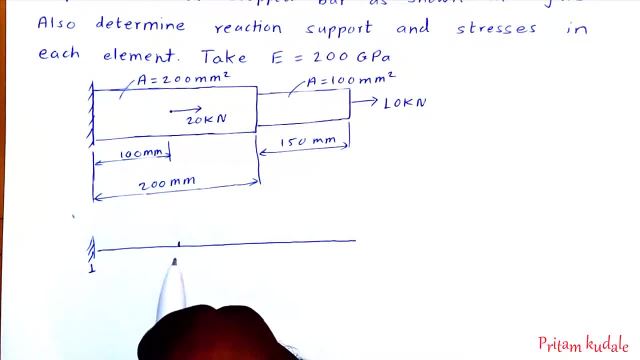 be your node 1, then at the point load it is node 2, at the change of cross section it is node 3 and at the end it is node 4.. And element numbers you are going to write in a simple circle. so 1st element, 2nd element, 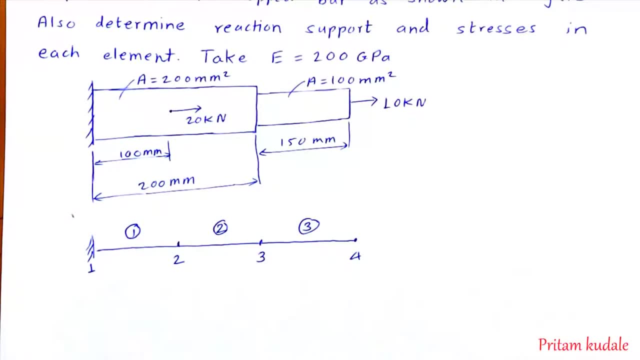 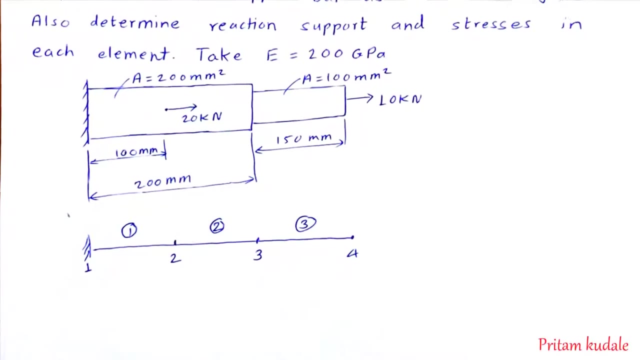 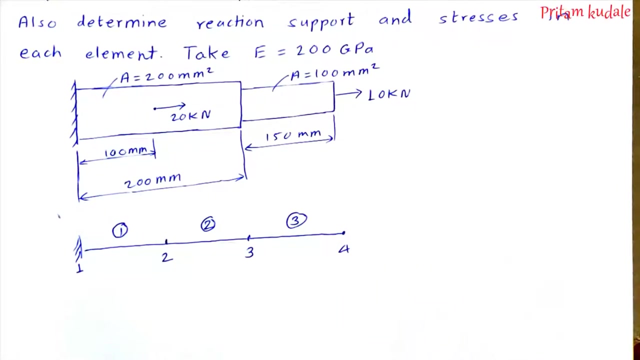 and 3rd element. So this is the conversion of real life problem into the analytical problem. So here, Whatever, the at each node will be denoted by D and the force is denoted by letter F. Now, after this discretization process, we have to create a element: connectivity table. 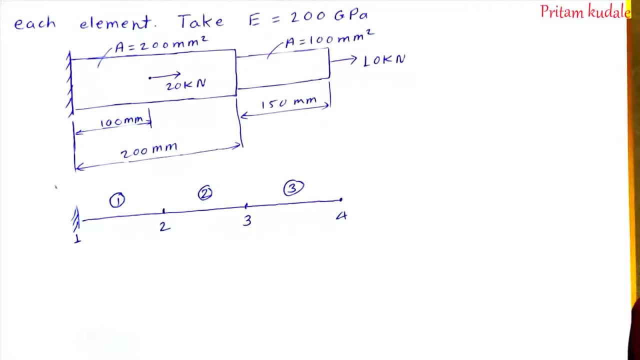 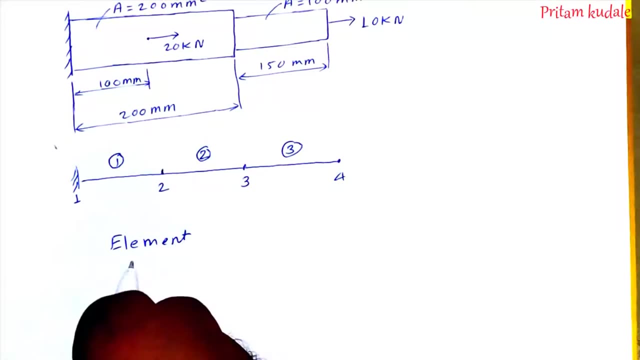 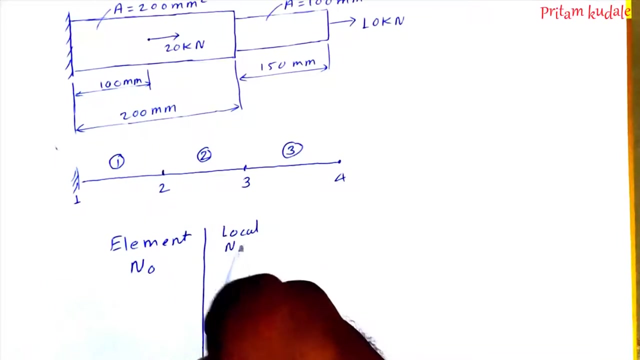 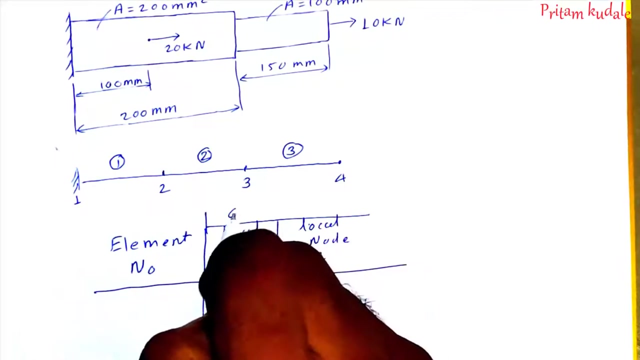 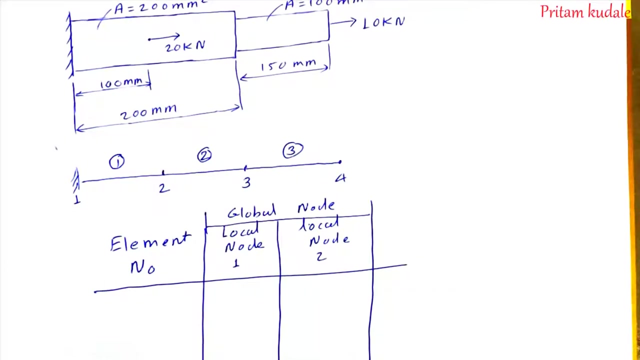 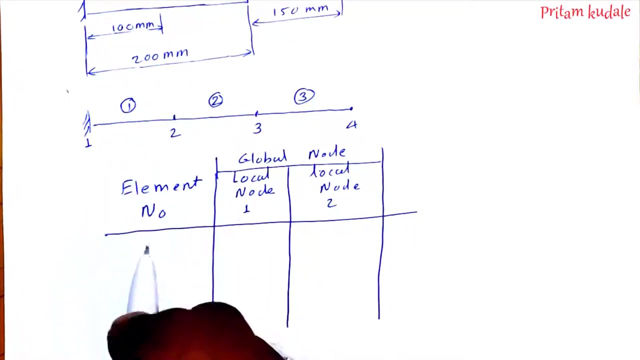 so for element connectivity table, we are going to write first element number, then local node 1 and local node 2.. and element: we are going to write its global node that we are going to represent in this table. So for element 1, you can see over here, this is the element which is in the circle, so that 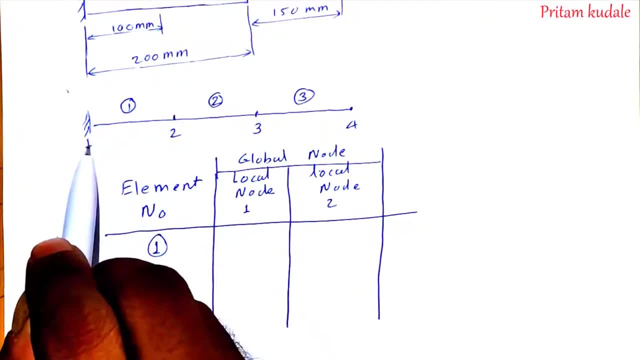 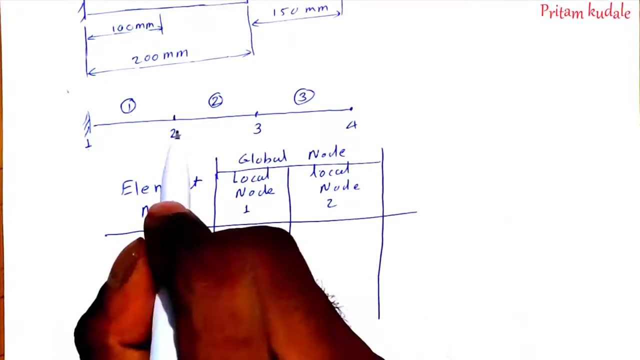 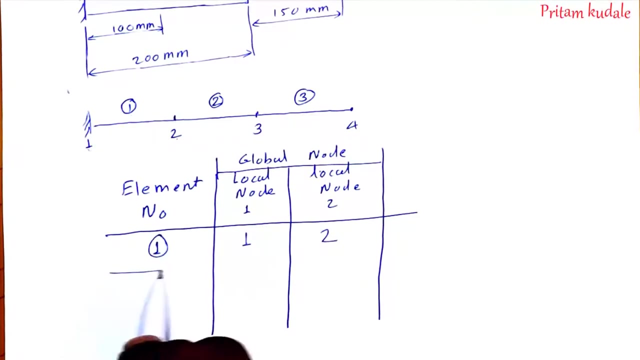 is the element 1 having the connectivity. left hand side is for the 1 and right hand side 2, so its local node 1 will be 1, local node 2, which is having value 2.. So this is our connectivity of first element. then we are going to check connectivity for. 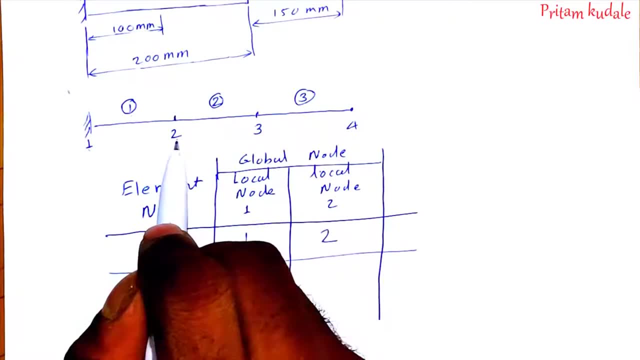 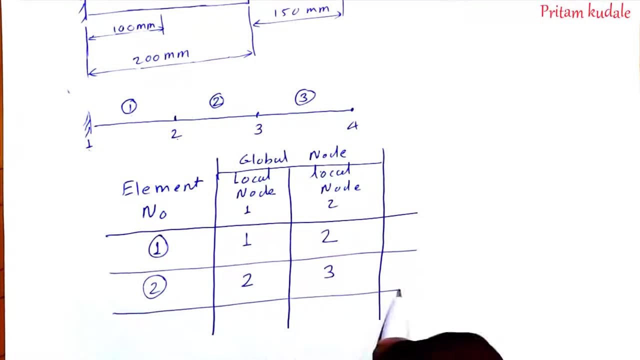 the second element. so in second element, left hand side value is 2, right hand side value is 3, so it will be 2, 3. and for third element, left hand side, you can see it is 3, right hand side 4, so 3, 4. so as long as your element connectivity is straight forward, this value. 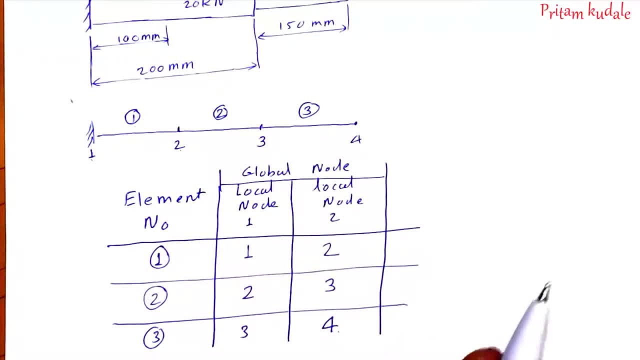 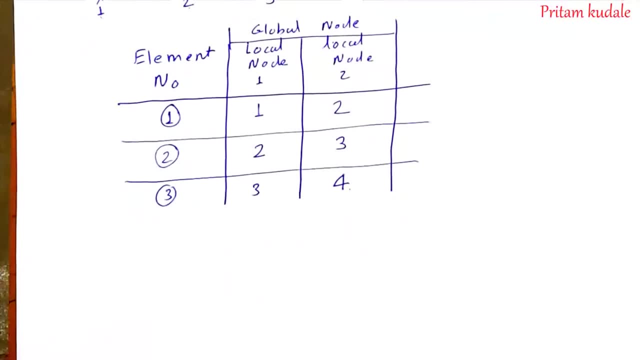 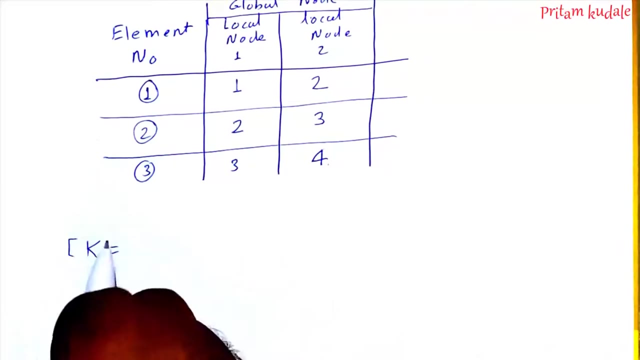 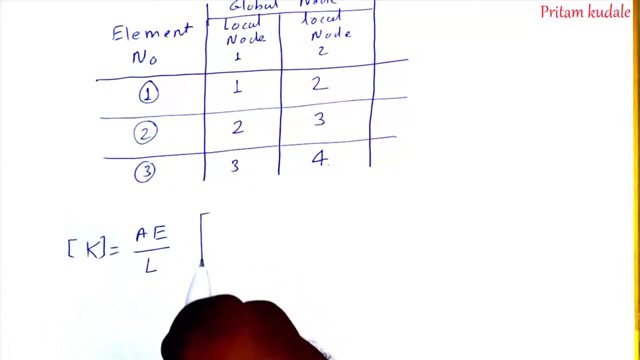 will be straight: 1, 2, 2, 2, 2, 3 and 3, 2, 4. ok, Now, after that, we are going to proceed with the stiffness matrix. so in stiffness matrix for 1D, 2 Noded formula, we know the matrix that is, the K is equal to AE by L and connectivity. 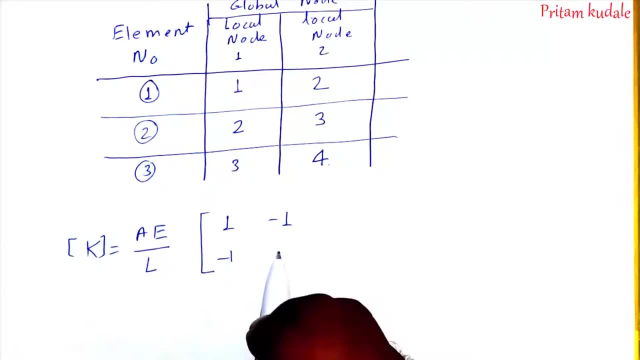 will be 1 minus 1 minus 1 and 1.. So 1 D, 2 Noded formula. we know the matrix, that is, the K is equal to AE by L and connectivity will be 1 minus 1 minus 1 and 1.. 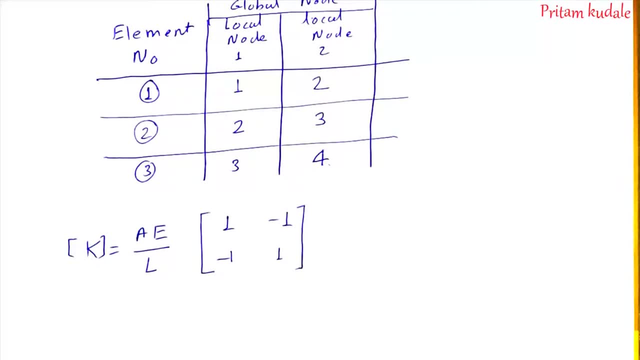 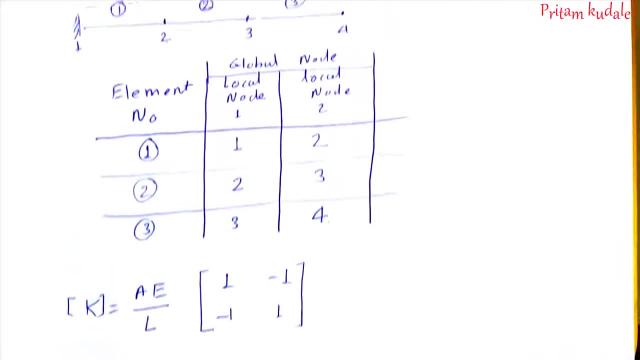 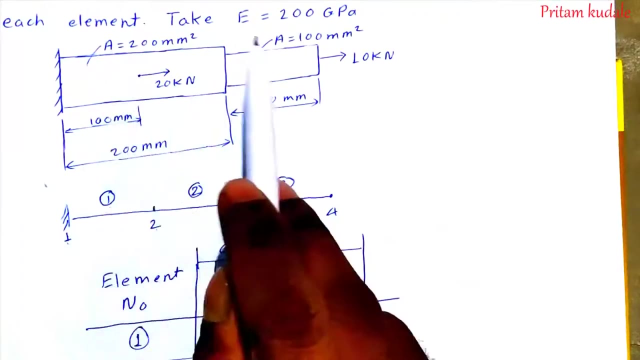 So this is your general local stiffness matrix formula for 1D 2-noded 1D element. Now for the given diagram. we have to write down what is the area. So for first element, area is given. 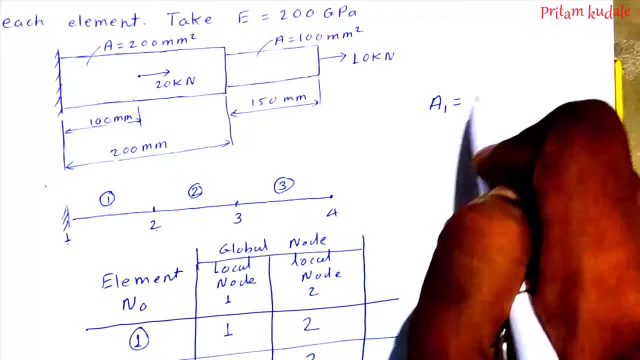 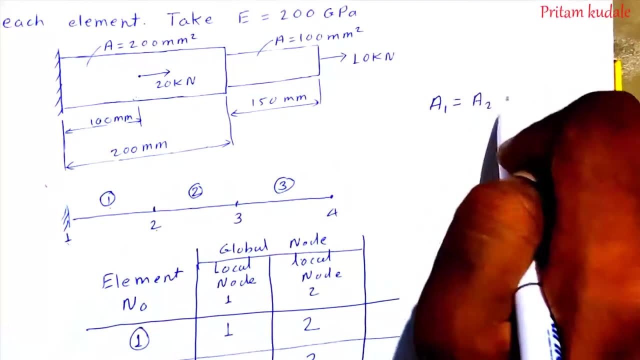 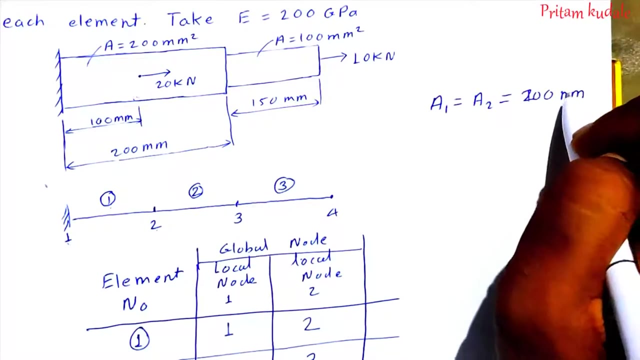 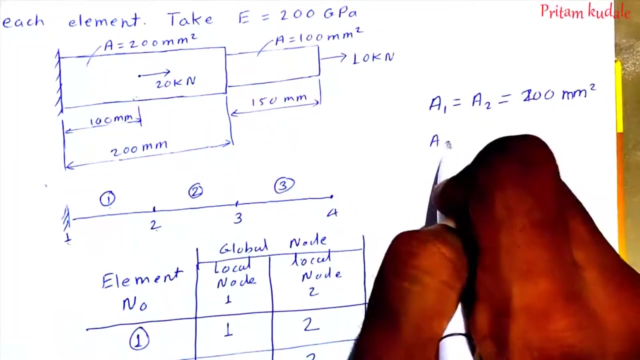 I am going to write it over here: Area A1 is same as A2.. Whatever second element having the same cross-section area- So A1 is equal to A2- is equal to 100, 200 mm square. Okay, Then for third element, A3 is having 100 mm square. 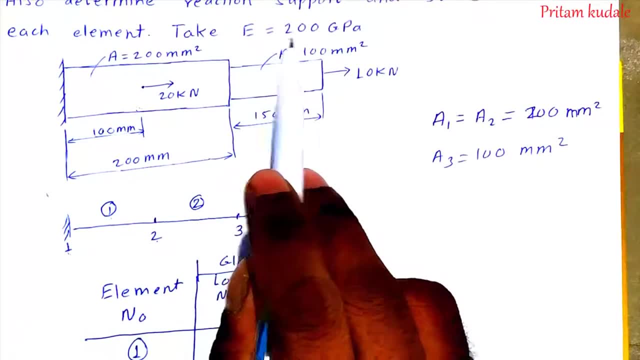 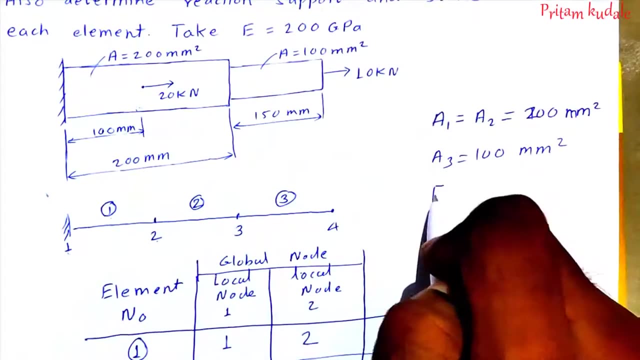 Now in the question it is given that E is equal to 200 GPA, which is common for all the element. So we are not going to separate it as E1, E2, E3, all. we will take it as a 200 GPA. 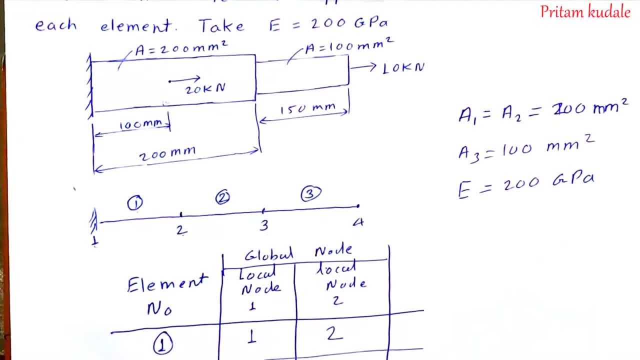 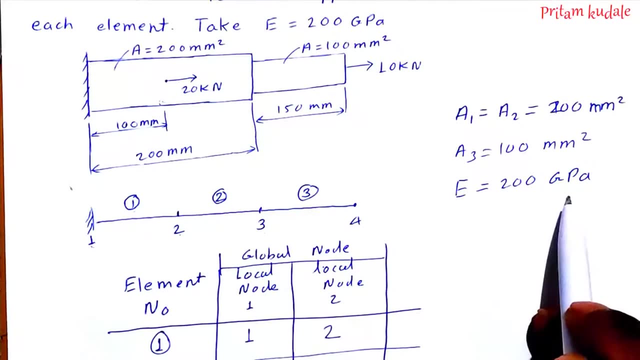 Now we have to convert. all things should be in Newton and mm. So for GPA you are going to convert it into MPA. MPA is equivalent to Newton per mm square. So we are going to convert it as 200 into 10, raise to 3.. 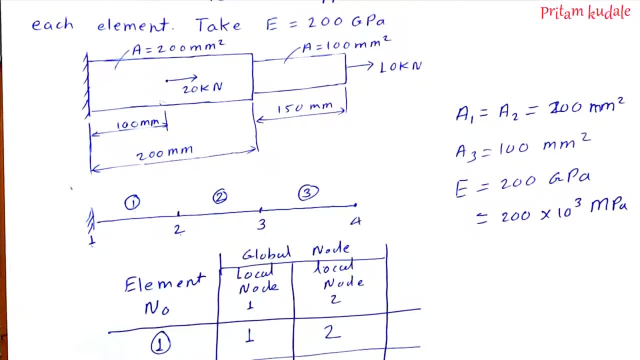 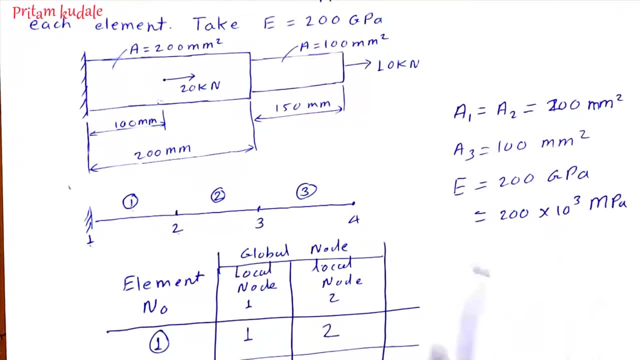 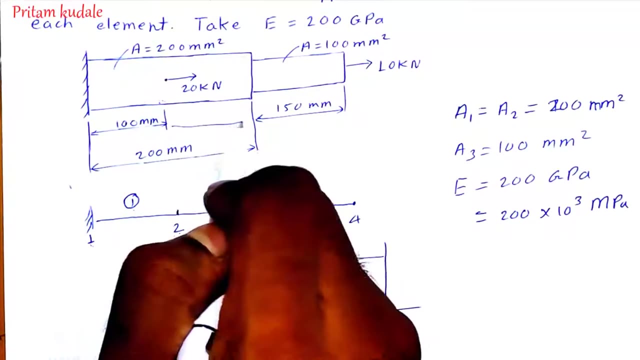 MPA, which is nothing but Newton, per mm square, and that's this we are going to use for our calculations purpose. Okay, And length in length. Also, this length is given as 100 mm. So again, this length, 200-100.. 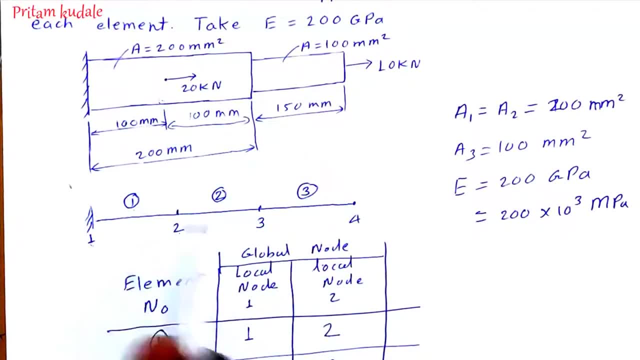 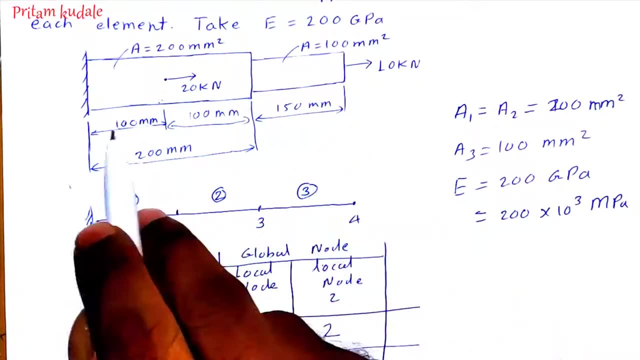 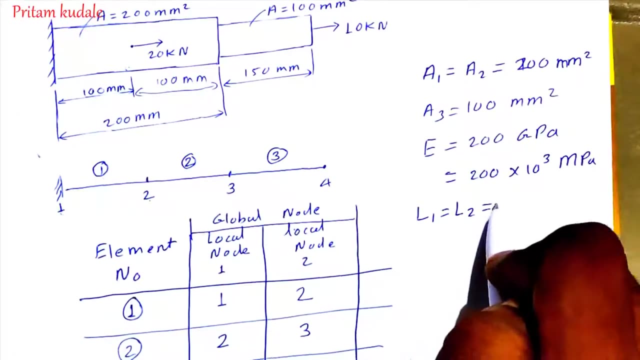 So it will again come to be 100 mm. So length of node 1 as well as node 2, element 1, element 2 and element 2 are equal to 100.. L1 and L2 are same. so that's what I am going to write again. L1 is equal to, L2 is equal. 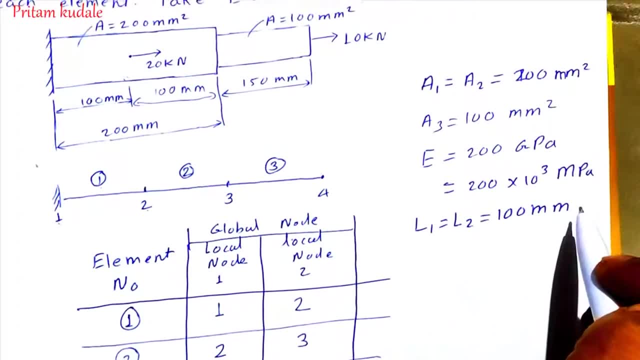 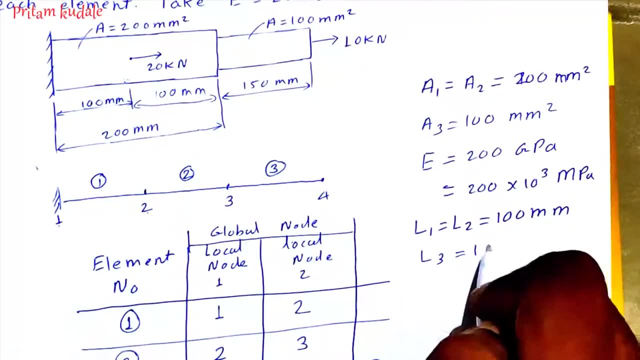 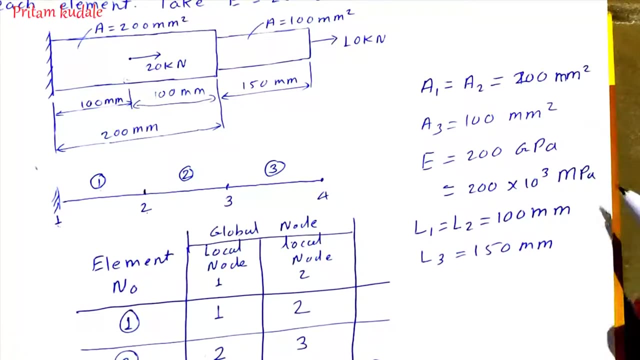 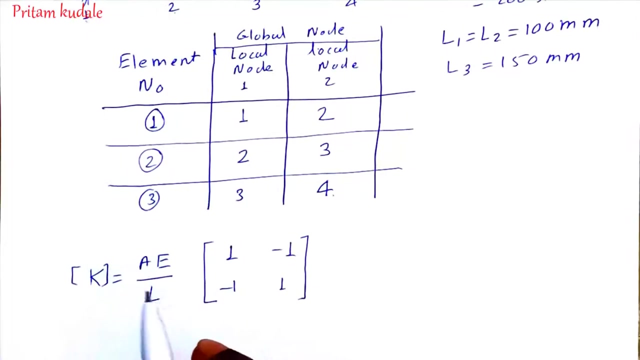 to 100 mm and L3. for node 3, the length is different, that is 150 mm, so L3 is equal to 150 mm. now all our units are Newton per mm square form, Newton and mm form. so let's come back to the equation now, in this particular equation, to calculate the K1. so I am again. 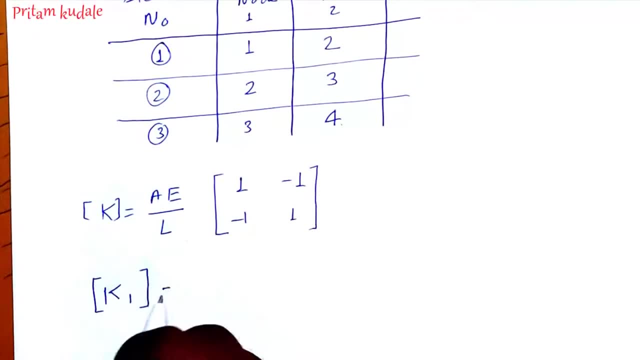 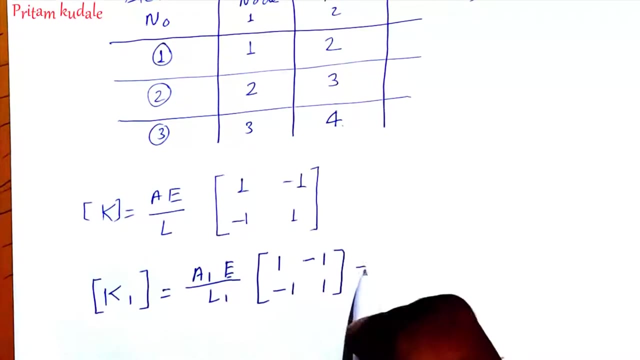 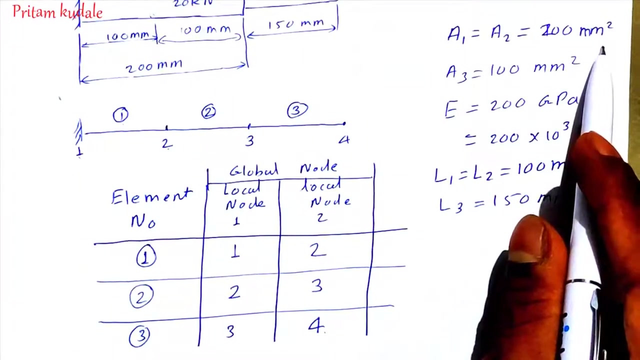 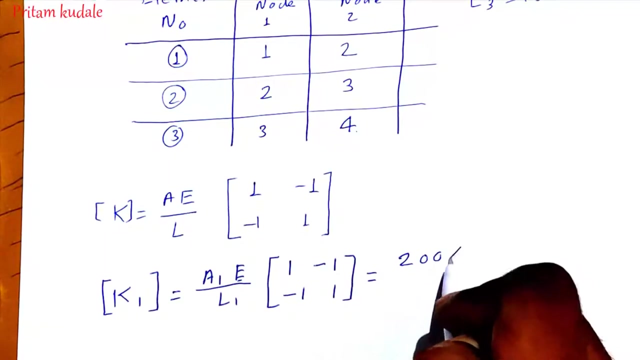 going to repeat it for calculating of K1. it will be: a1- E is common, divided by L1 into 1 minus 1 minus 1, 1. now put the values. so, first of all, the value of A1 is 200 mm2.. So value of A1 is equal to 200 mm2. into E, E is given as 200 GPA. that 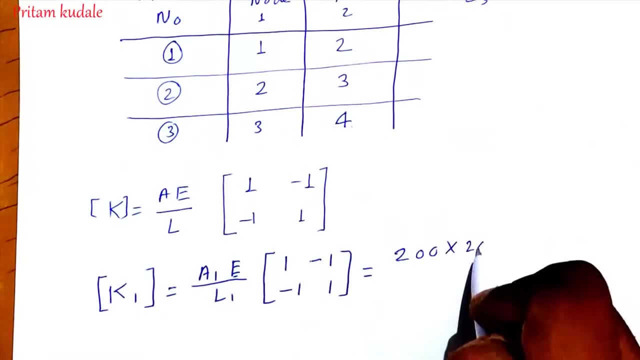 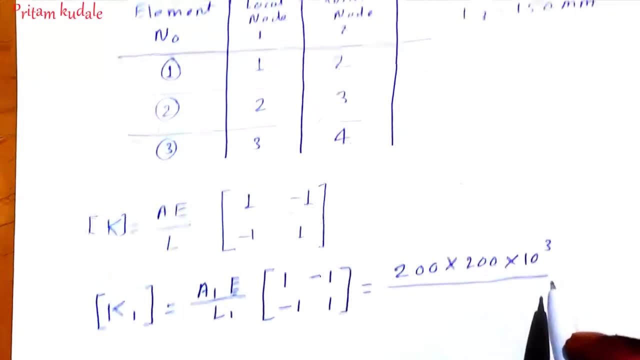 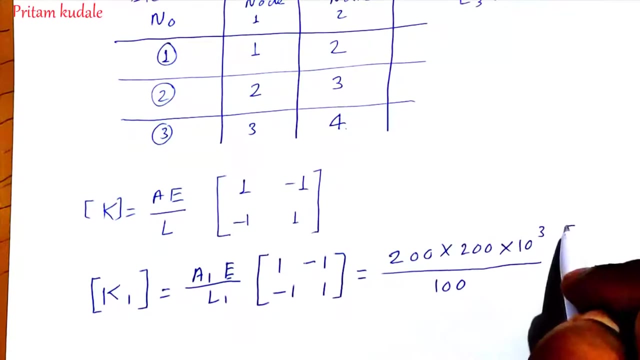 is 200 into 10, raise to 3.. So into 200 into 10, raise to 3, whole divided by length. Length is given as 100 mm. So divided by 100 and again multiplied by 1, minus 1, minus 1 and. 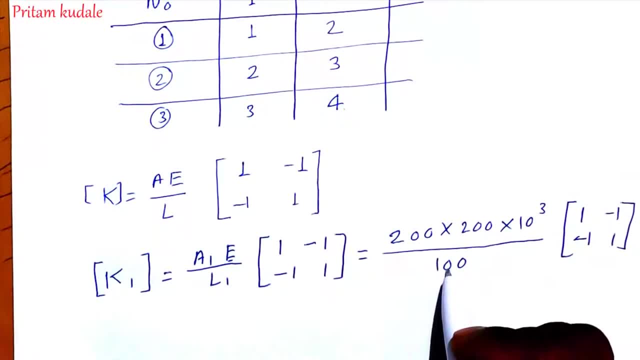 1.. So if we consider this will get cancelled, this 2 will get cancelled. Then 10 raise to 3, if we multiplied it by 100, it will be 10 raise to 5.. And what will remain here? 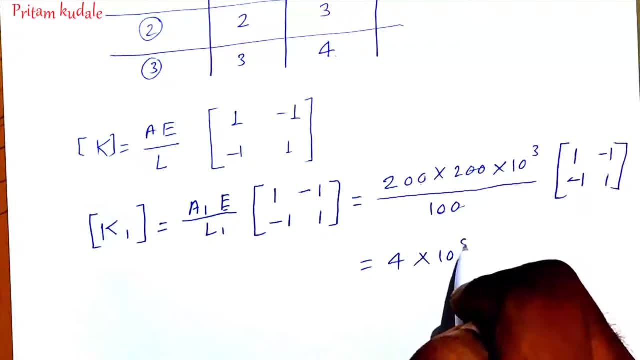 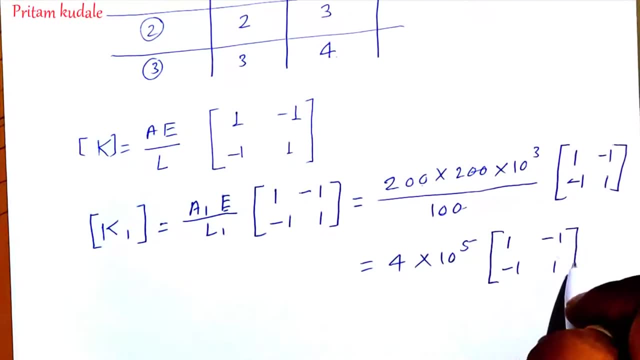 That is, 4 into 10 raise to 5.. 1, minus 1, minus 1, 1.. So in all three elements, 10 raise to 5 will be a common factor which will remain outside the bracket. So that's why we are going to put some common factor. 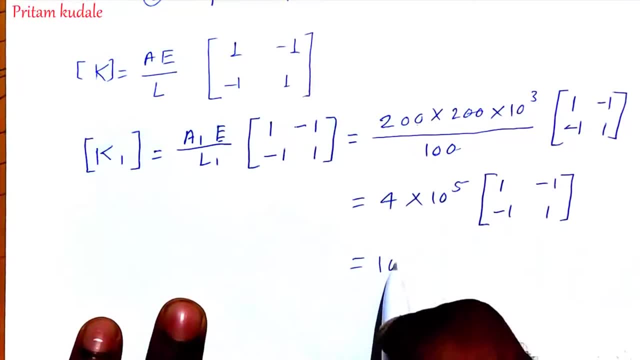 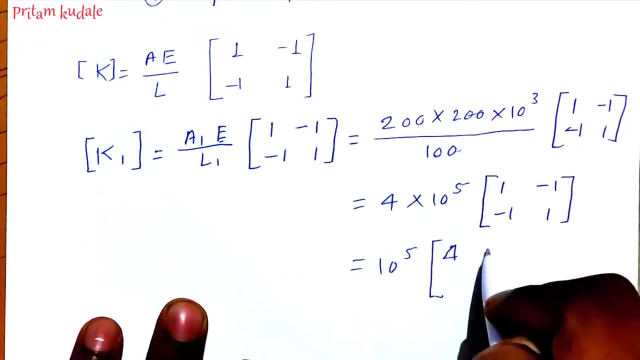 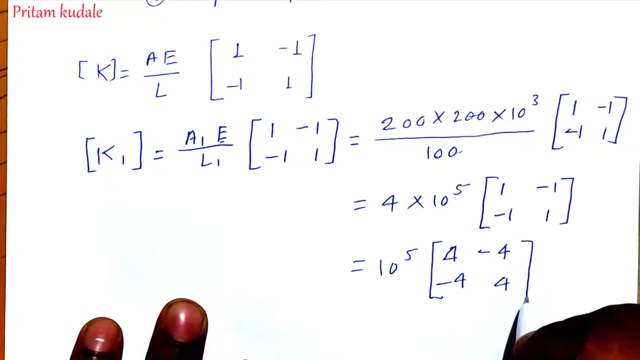 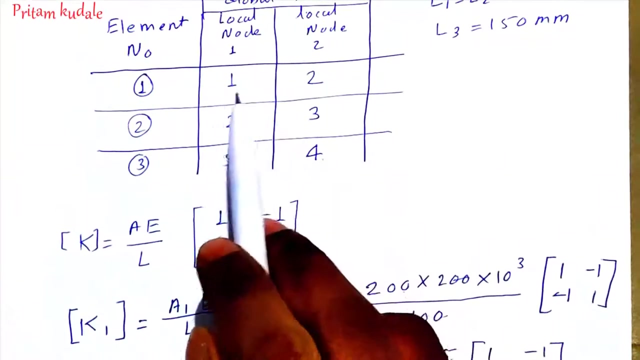 inside the matrix. So we can write it as: 10 raise to 5 into: when 4 multiplied by 1, it will be converted to 4. Minus 4. minus 4 and 4. so this will be our converted matrix. now from connectivity table we are going to write: 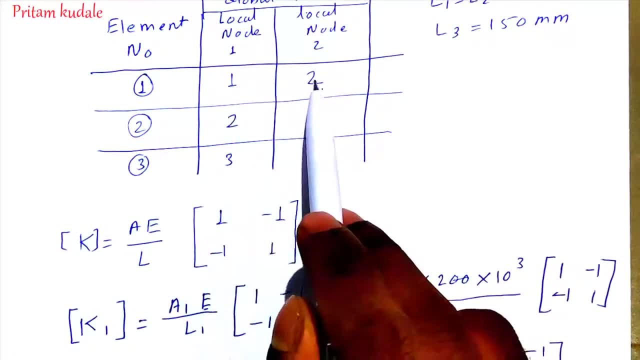 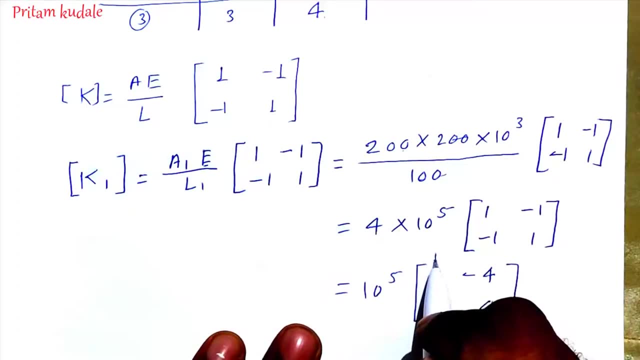 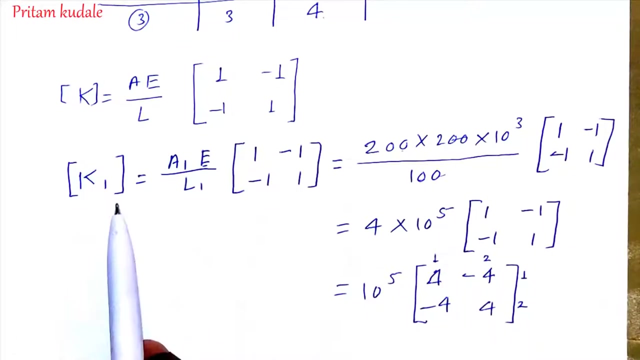 down its connectivity. so what is its connectivity? 1 to 2? the same. we are going to rename its column as well as row, so your column is 1 and 2. similarly, row we are going to rename as 1 and 2, so similarly, we are going to repeat the same procedure for k2 as well as k3. now, if we consider: 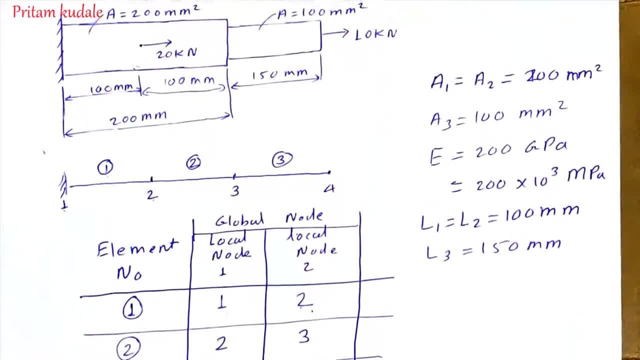 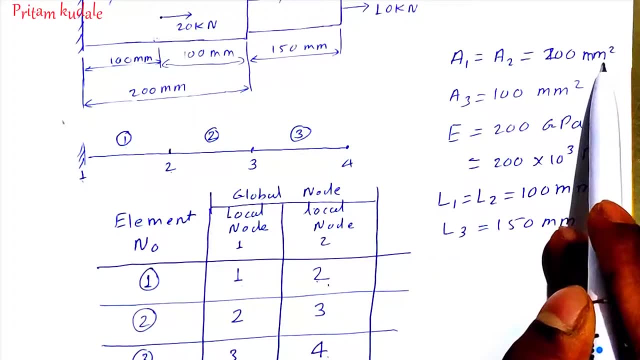 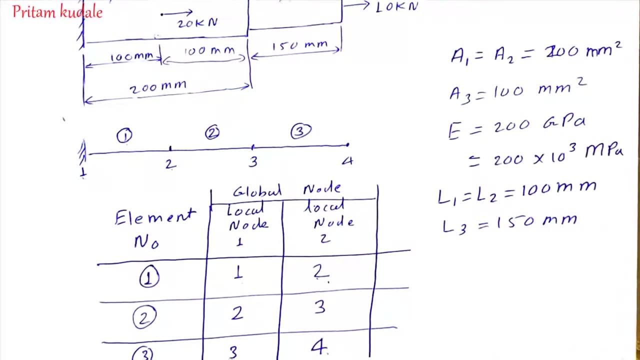 our value of a1 and a2. both are same 200 mm square, then E is common for all, as well as L1 and L2 are same. that is 100 mm Square. so if we come to this particular formula, a1 and a2 are same, e is same, l1- l2. 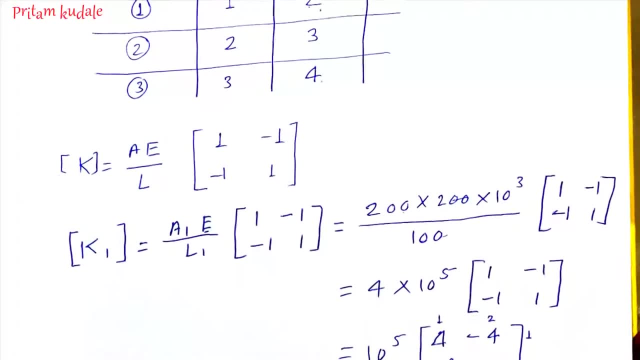 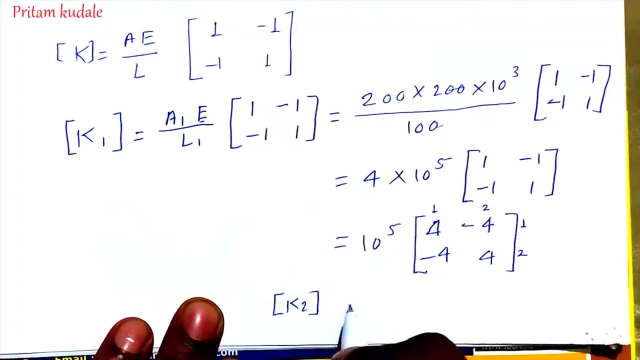 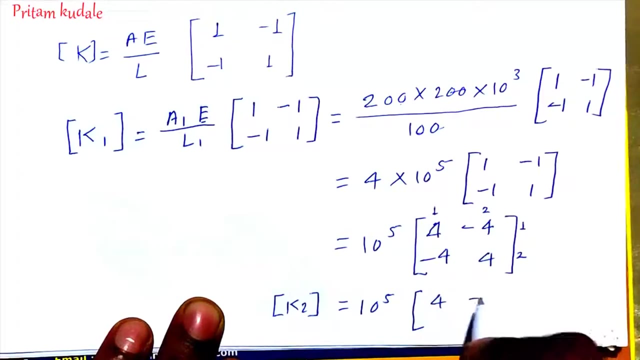 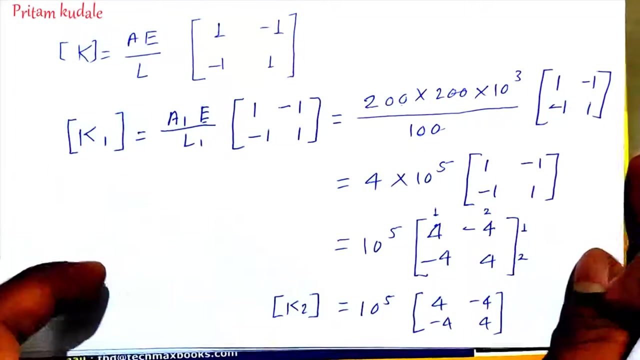 are same. so our k1 and k2 will be same. so the value of K2 will be same: 10, 0, 10. 10 to 5 into bracket 4 minus 4 minus 4, 4. but what will be change the connectivity? 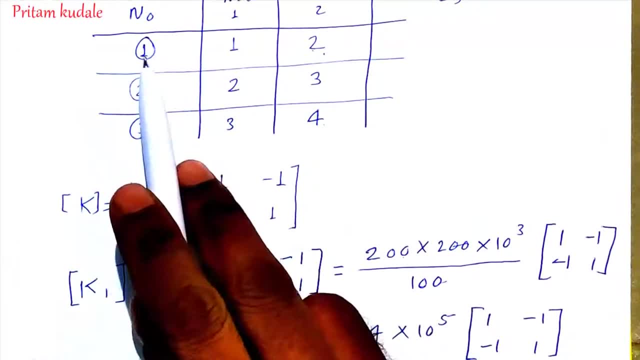 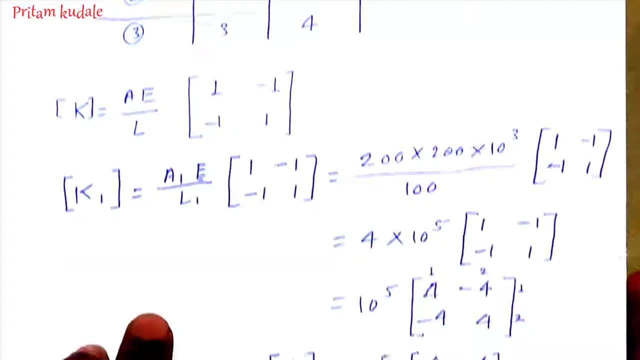 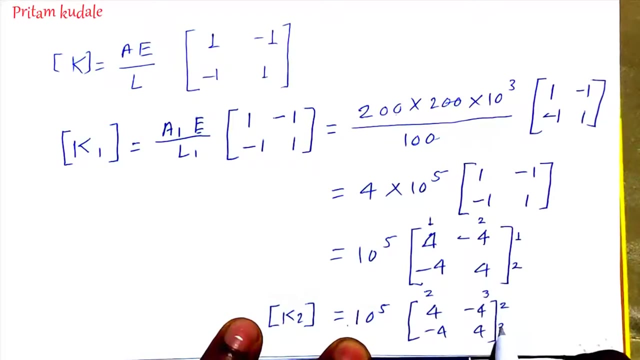 for node 1, element 1, connectivity is 1 to 2. for element 2, connectivity is 2 to 3. so that's what we are going to write: connectivity as 2 to 3 and 2 to 3. and now we are going. 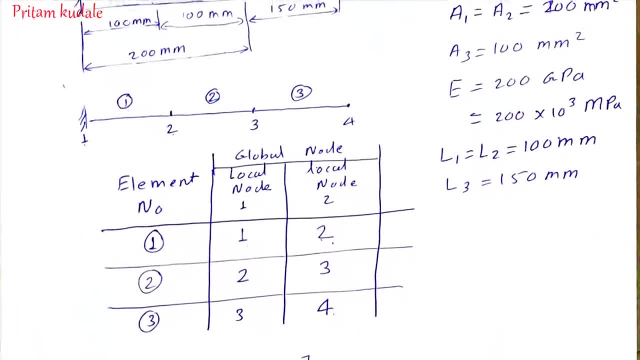 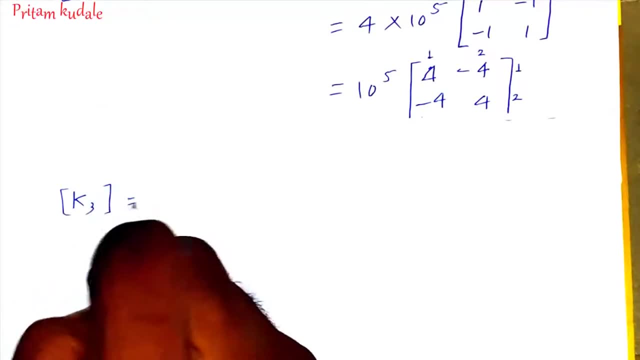 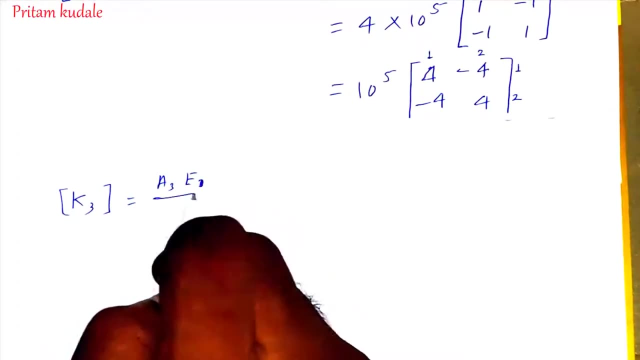 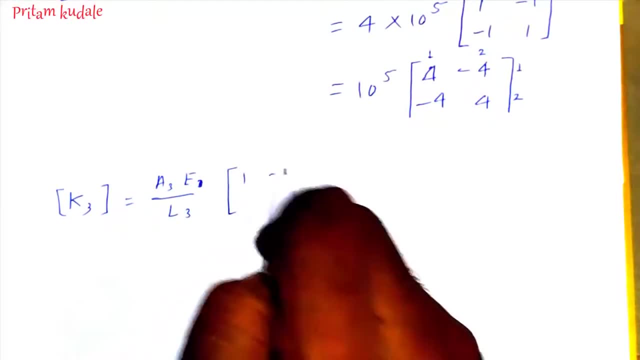 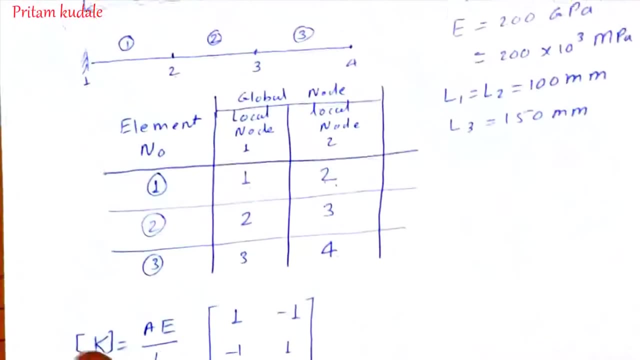 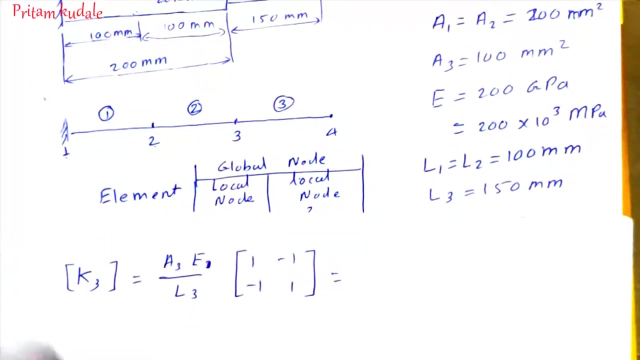 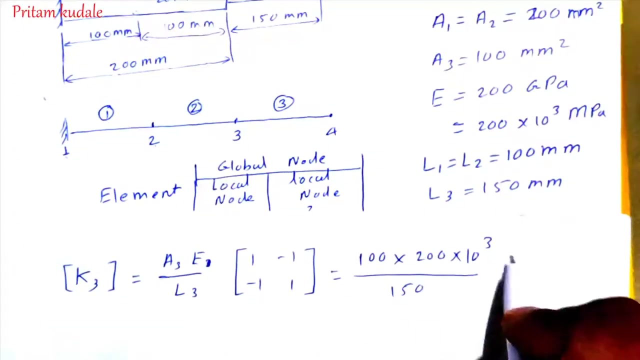 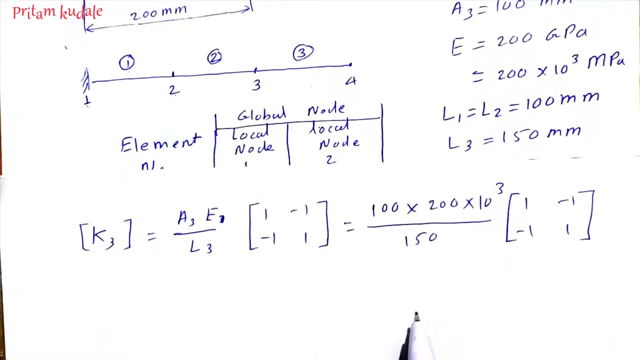 So K 3 is equal to a 3. E is common divided by 2.. K 3 is equal to a 3. E is common divided by 2.. that is 150 into 1 minus 1 minus 1, 1. so k3 will be 1.33 into 10. raise to 5, so you have to keep. 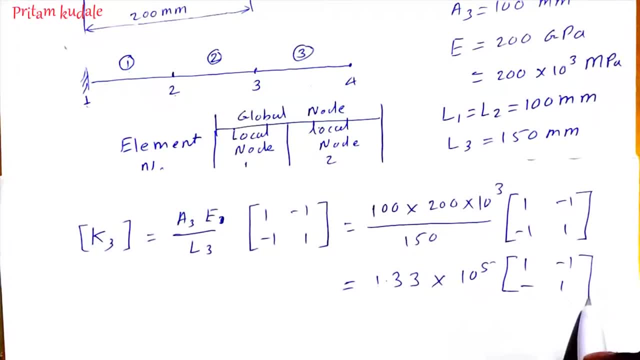 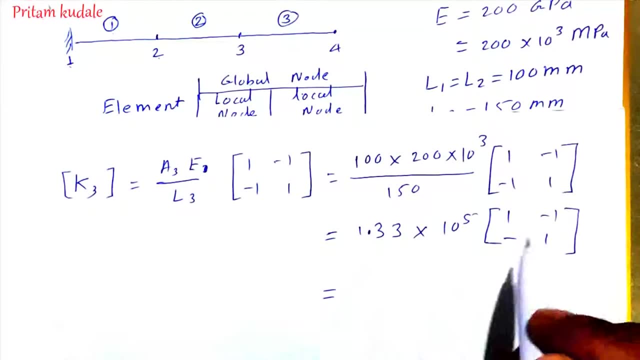 this factor common. so 1 minus 1 minus 1, 1 and you are going to convert it, you have to put 1.33 inside the bracket. so 10 raise to 5, that is a common factor. and 1.33 minus 1.33 minus 1.33. 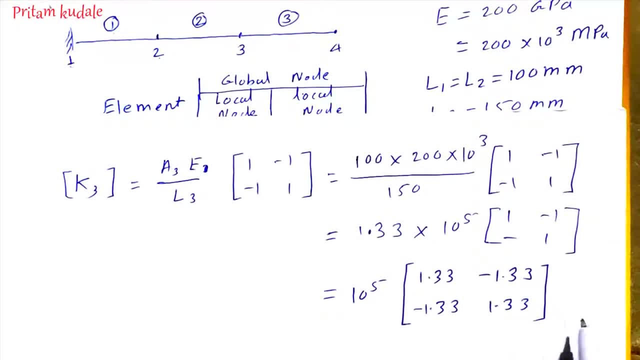 and 1.33, and then you have to write the connectivity. so its connectivity for third element is 3, 2, 4. so 3, 4, 3, 4 that you have to write now. after this local stiffness matrix you are going to form a global stiffness matrix. so first, 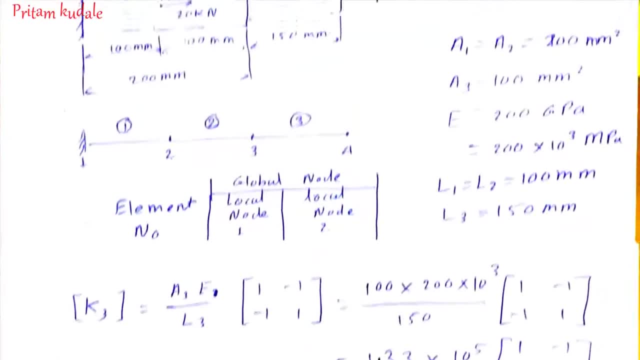 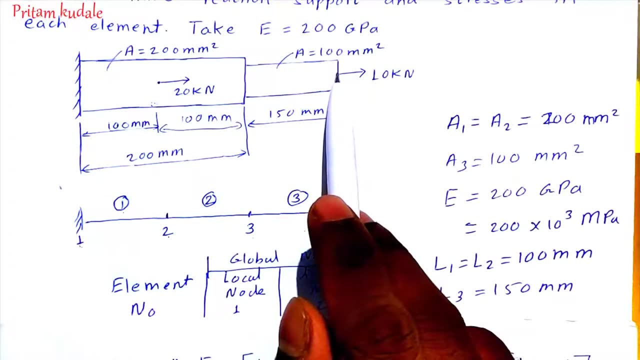 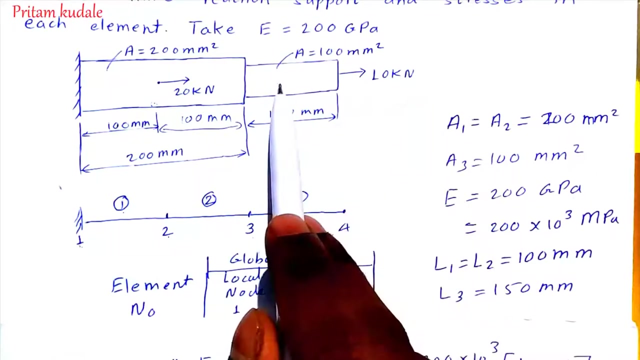 of all, you have to decide what should be the dimension of global stiffness matrix. so according to this particular numerical, as it is a 1D element, the degree of freedom for each node is 1, because this element can only move in X direction, that is, in rightward or leftward direction, but movement in other 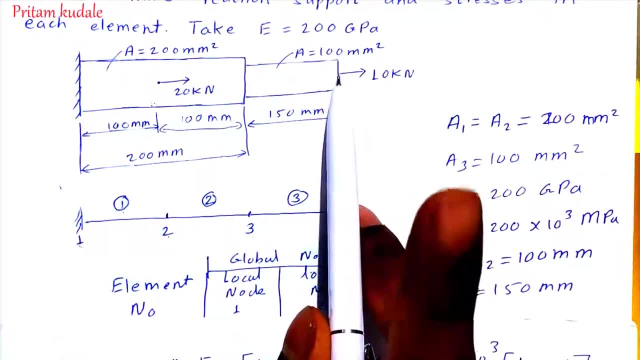 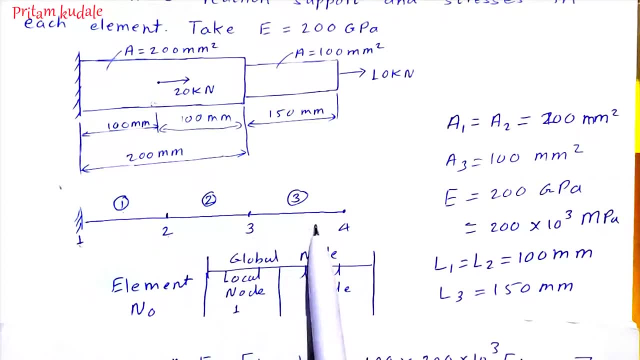 two direction are blocked. so degree of freedom of this node is only 1. so to decide the size of the global stiffness matrix it will be the number of nodes into your degree of freedom for each node. so as the degree of freedom for each node, the total number of nodes are 4. so 4 into 1, 4, so your size of global. 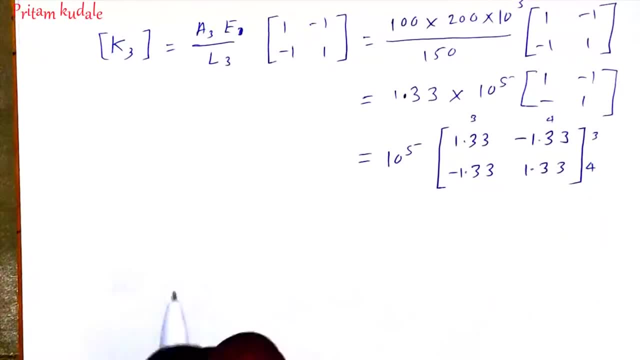 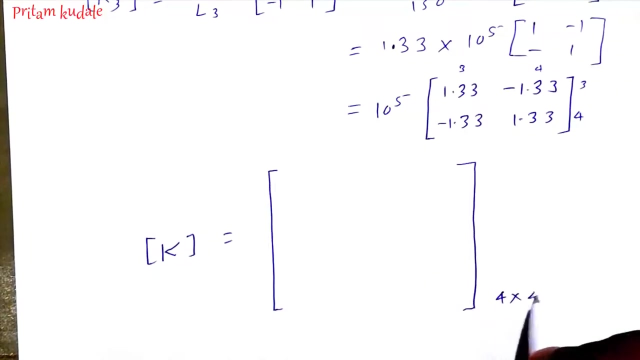 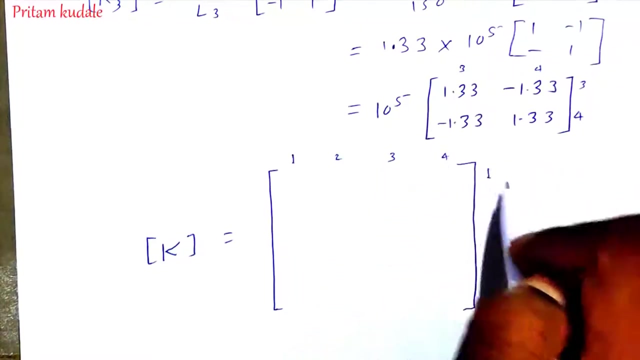 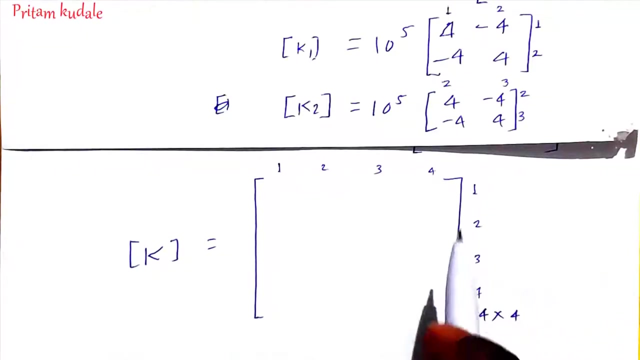 stiffness matrix will be 4 by 4. so you have to write your global stiffness matrix: K is equal to. so you have to take a matrix equal to 4 into 4 and you are going to name the column 1, 2, 3, 4 similarly: 1, 2, 3 and 4. now to add the local stiffness matrix into. 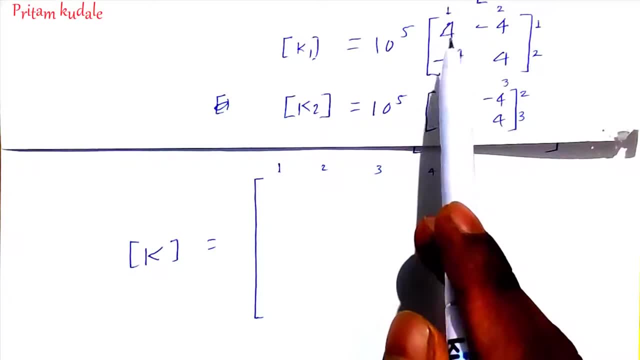 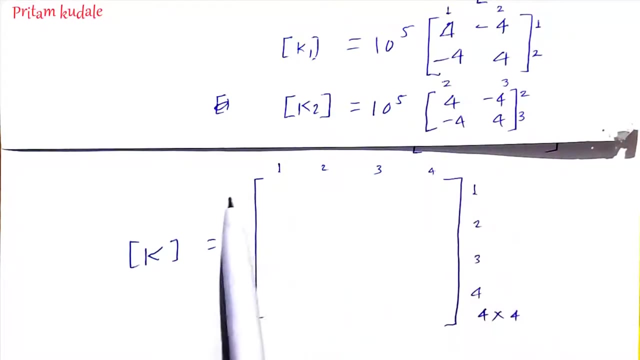 the global stiffness matrix you are going to use equate the row number and column number of both the matrices. so in for adding the K 1 first, we will add the first value, which is having the first column, first row. having the value 4, we are going to add it here first, row, first. 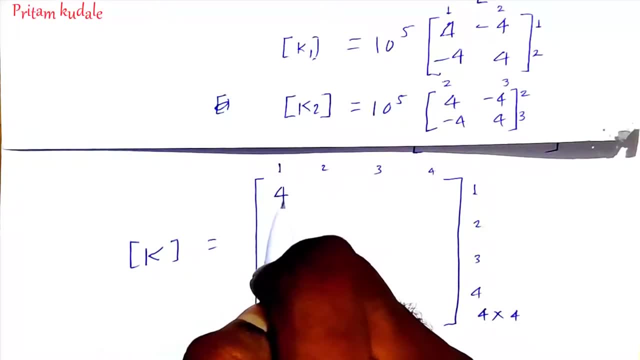 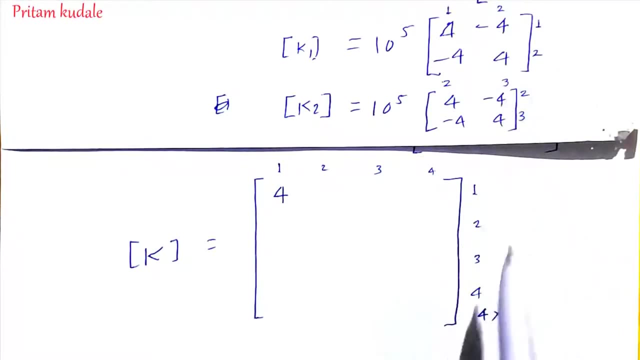 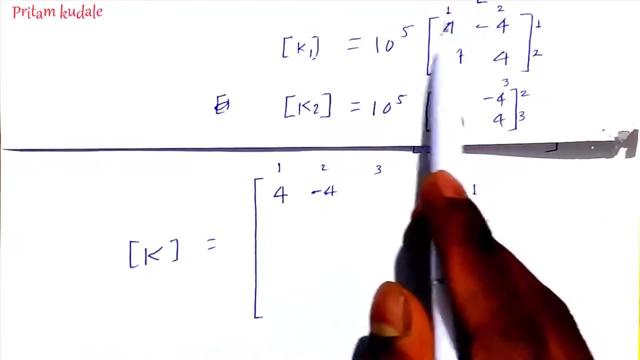 column value 4. we are going to write it over here. then for second column, first row, so first row, second column, value is minus 4, same. we will write first row, second column as minus 4. then first row is completed, we will jump to the second row. so second row, first column having the value of: 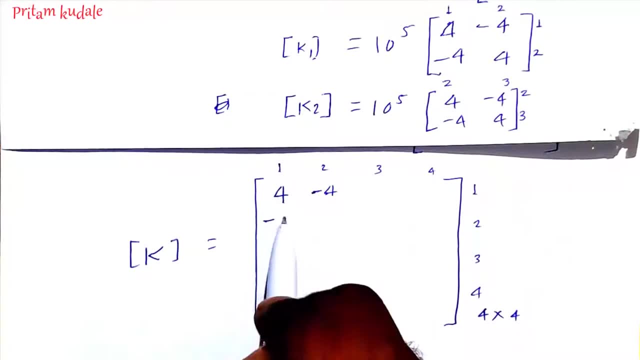 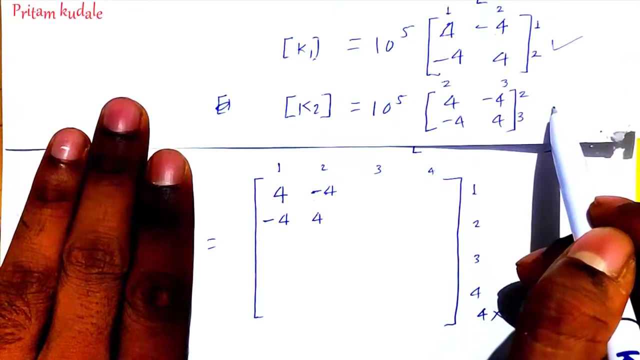 minus four. so second row, first column, you are going to write the value of minus 4. then second row, second column, value is plus 4, so that what we are going to write. so our first K1 matrix is completed. now we will add the K 2 matrix. so for K 2 matrix it start with the second row. 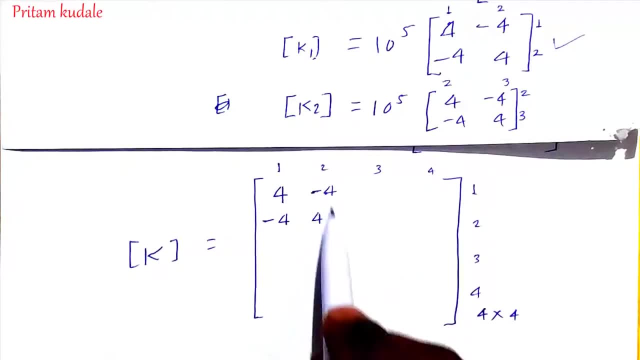 second column, so we will add it over here. second row. second row, second column. we already have one value, so we will add it over here, so it will come 4 plus 4. then second row, third column having the value of minus 4. so in global stiffness matrix, second row, third column having the value of minus 4. then 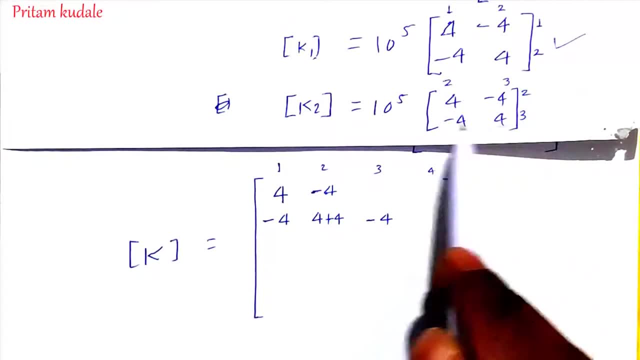 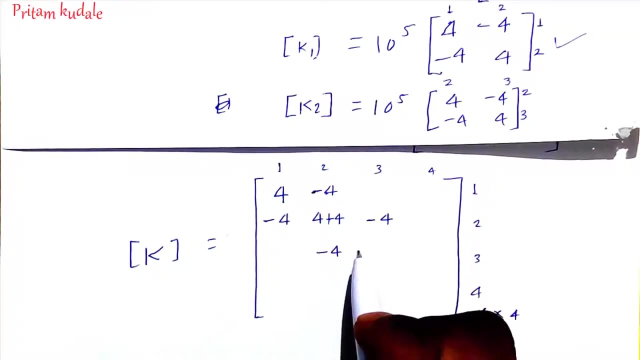 second row is completed, we will jump to the third row. so, third row, second column, minus 4. third row, second column having the value of minus 4. then third row, third column having the value of 4. third row, third column having the value of 4. 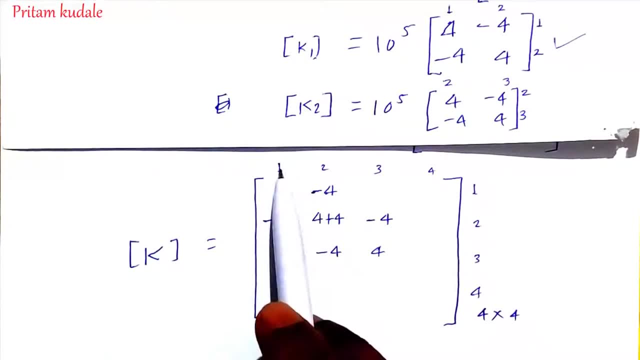 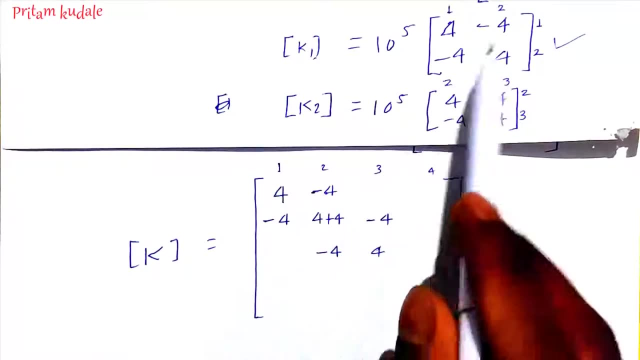 so you are here. you can observe that when the connectivity is straightforward, that is, 1 to 2, 2 to 3, you can directly write this particular box of the k1 matrices and you can directly write that is box into k2 matrices in between 2 to. 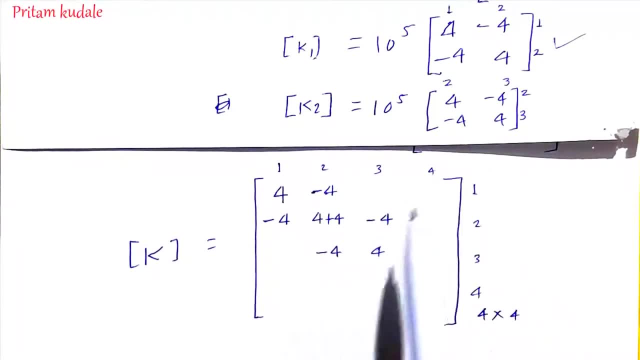 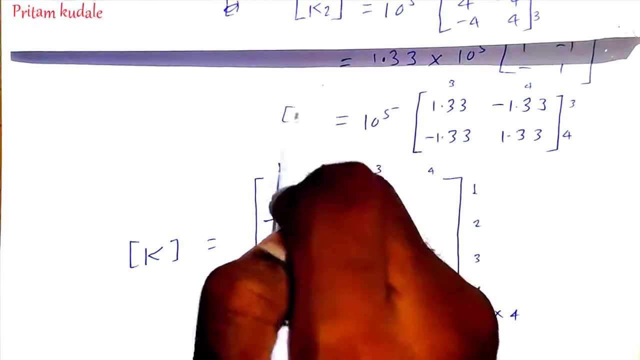 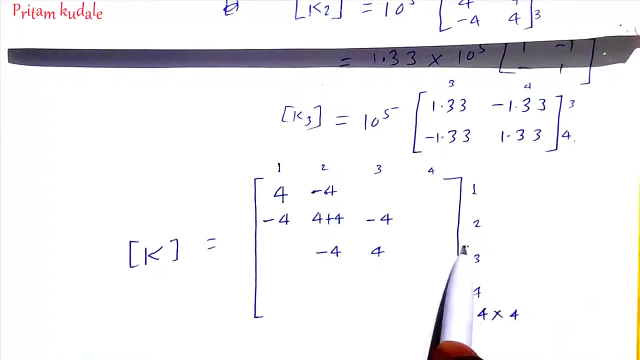 3 box, so second row and third column. you can directly copy it as it is. so if we referred it similarly for the third column, that is a k3 matrix, so in k3 matrix connectivity is 3, 4, 3, 4. so if we consider it over here we can directly. 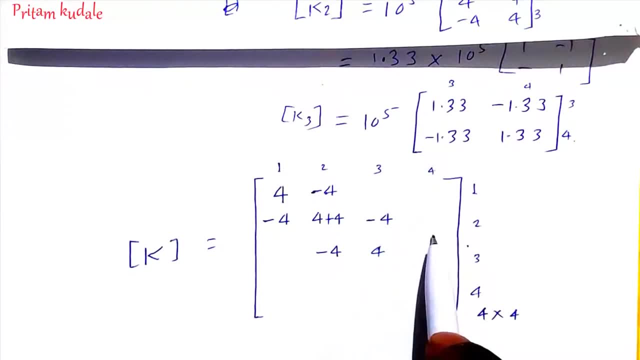 write it into the third and fourth row, third and fourth column, so this value is repeated. we can add it over here, so 4 plus 1 point 3: 3. so this value is repeated. we can add it over here, so 4 plus 1 point 3: 3, so 4 plus 1 point 3, 3. 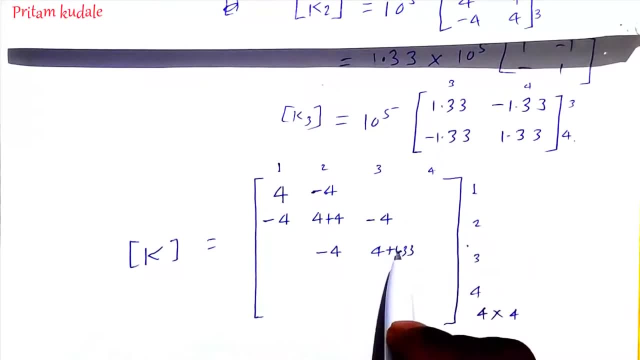 this value will be both value in 3 by 3 column and in next. we can write all this 3 value directly. that is, minus 1 point 3, 3, minus 1 point 3, 3 and 1 point 3, 3 over here now. now, whichever are the blank, you are going to fill it with the. 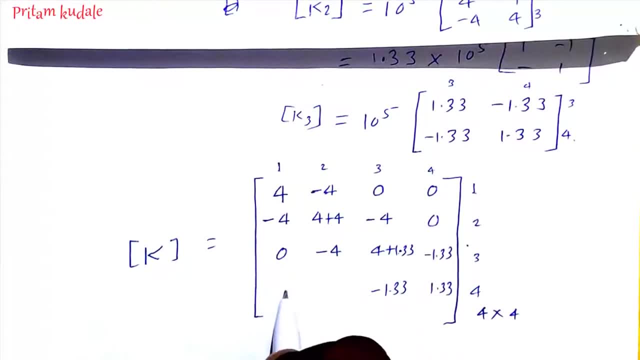 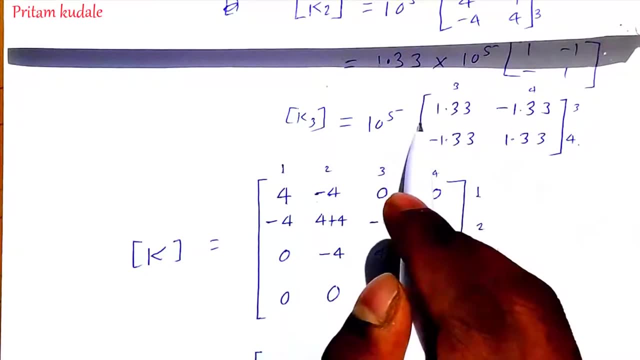 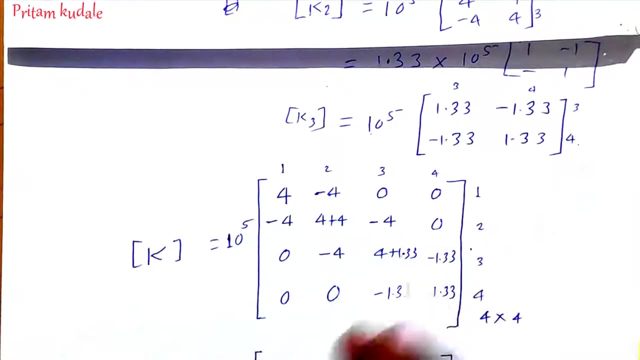 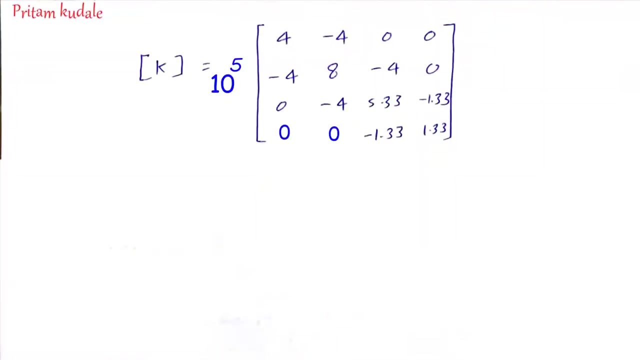 value 0. okay, staying the same, we will have Millionen's equation family and this will be the whole equation. okay, and now we will be saying that this equation is a global stiffness matrix and this will have any given expression. also right, and whatever the value that is outside the box will be repeated only. 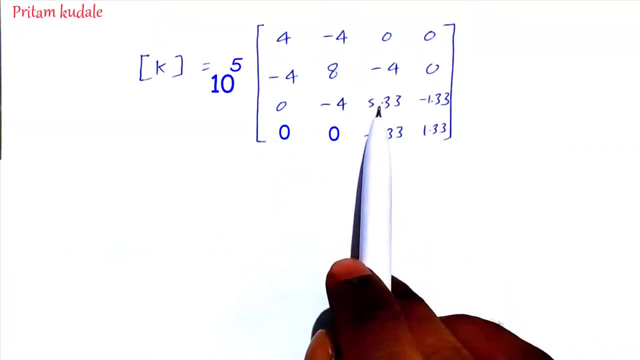 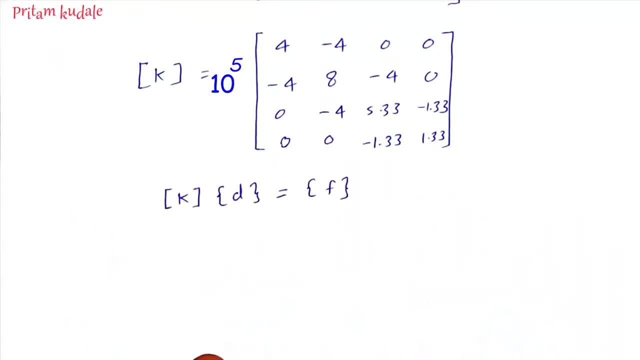 once. so 10 raise to 5 will be a common factor. you have to also take it here in a global stiffness matrix as a common factor. so after addition this will be: your global stiffness matrix is equal to F, where K stands for the global stiffness matrix, D stands for displacement. 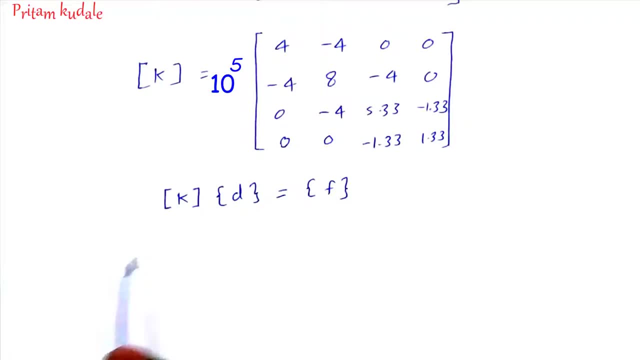 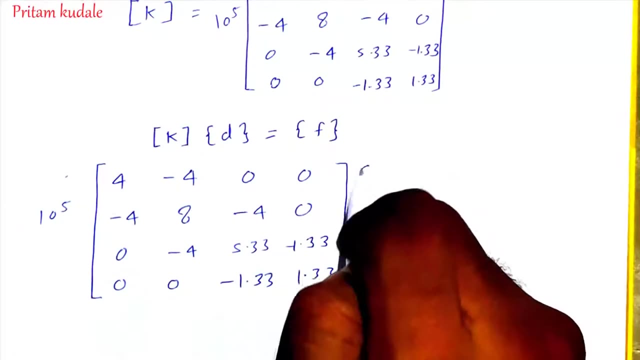 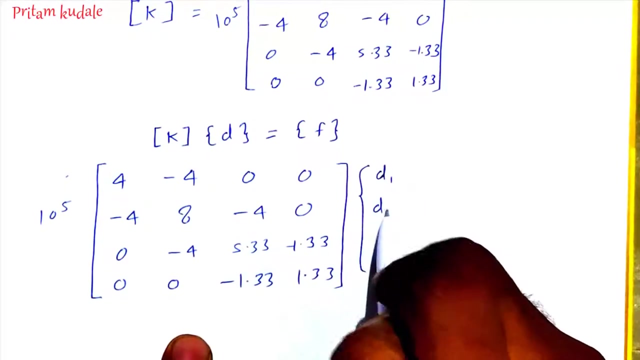 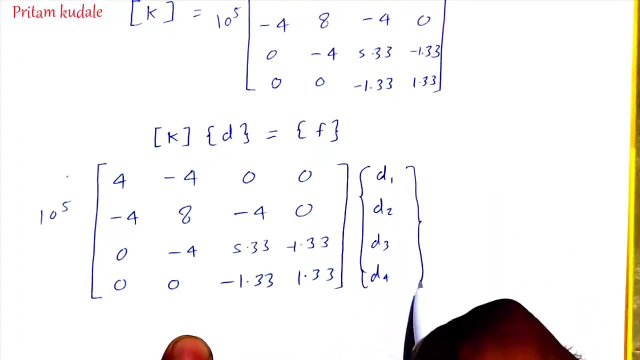 vector and F stands for the force vector. So same matrix will reflect over here. So this is your stiffness matrix, then multiplied by displacement. So for the first nodal displacement it will be D1, D2, D3 and D4. This will be your displacement of all 4 nodes. Then is: 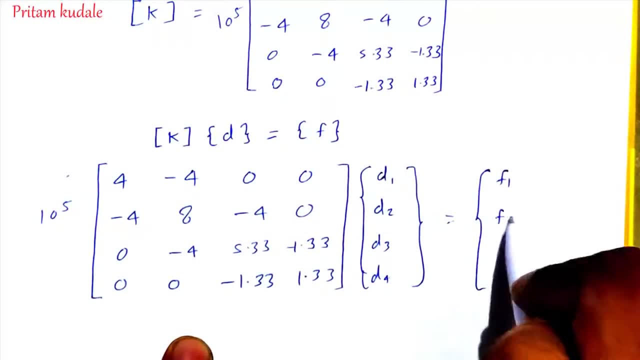 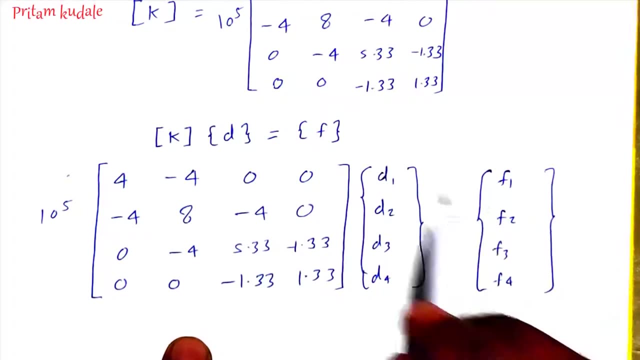 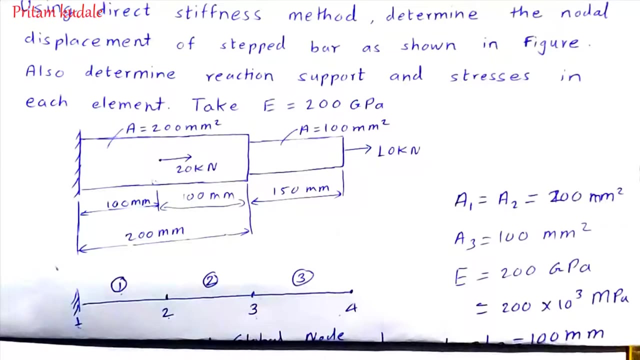 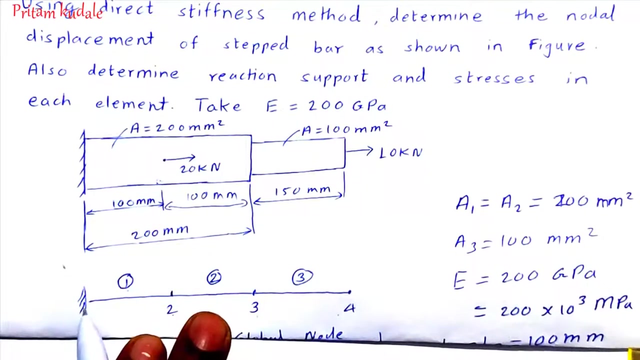 equal to your force, that will be F1, F2, F3 and F4.. So now we are going to put the value into this equation. Now, from this figure, we know that at the node 1 there is a fixed support. So this particular fixed support. 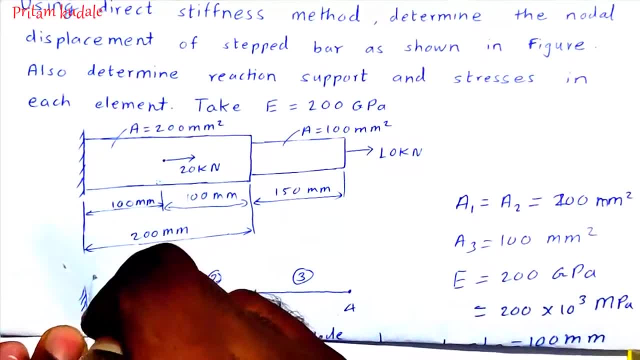 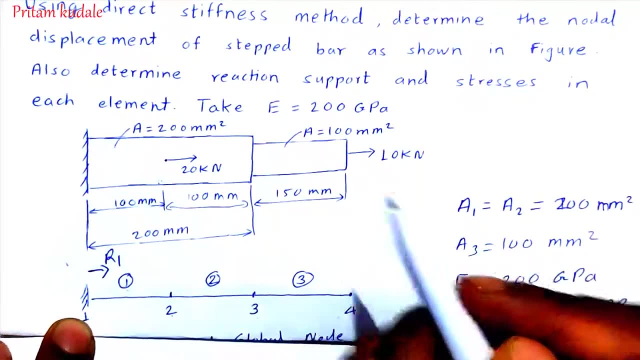 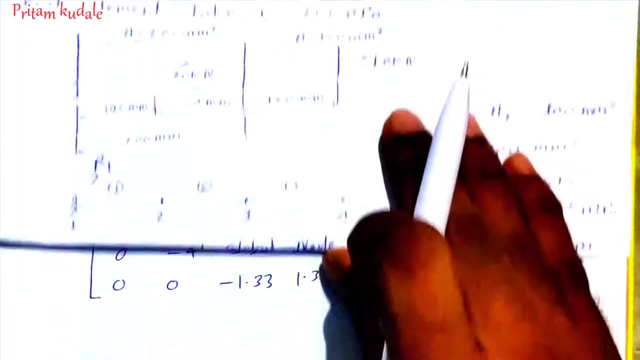 will create a reaction. So we will consider it will create the reaction in right side direction by the value of R1.. So we are going to always going to assume right side as positive and left side as negative. So we are considering R1 as in a right side. So we are going to. 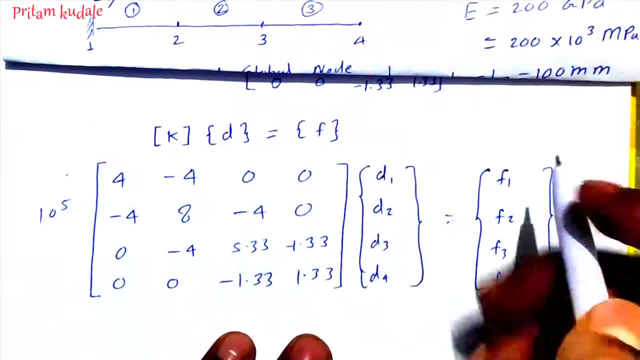 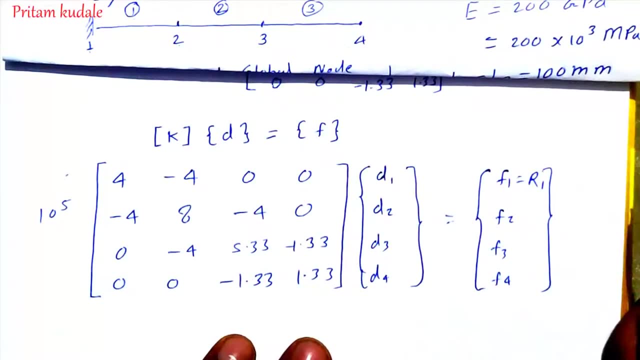 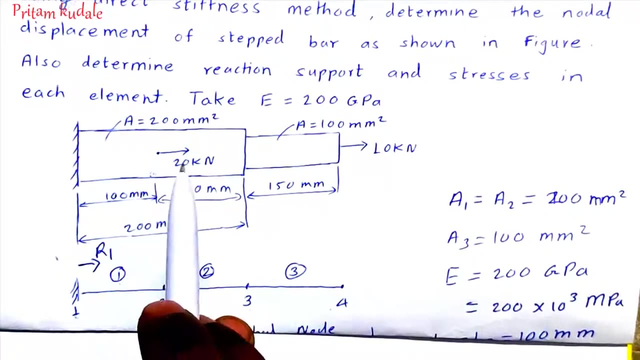 take it as a positive. So you are, F1 will be your R1.. So this will be, F1 will be your R1. Then you are going to write the F2 at the position of second node. your load is 20 kilonewton in rightward. 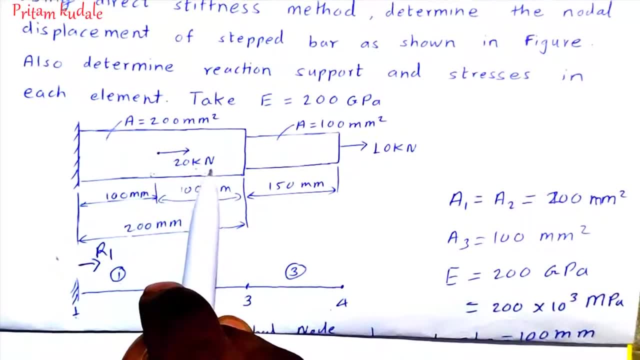 direction. So in kilonewton you are going to convert it into the Newton. So 20 into 10 raise to 3.. So F2 will be 20 into 10, raise to 3.. So if was the current load of F1, which was N2.. 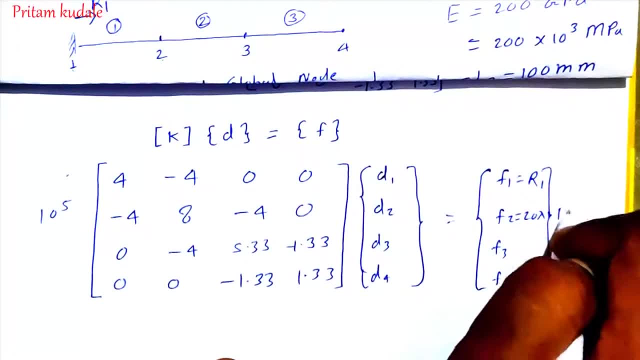 Okay now if you take 180 degrees forward at the time. so So the current load of F1 is 80 degrees and the operating amplitude 17 or 220 degrees. thereon is the current LPDH. So into 10 raise to the power 3, so it will be inside the bracket. so if this is a bracket, 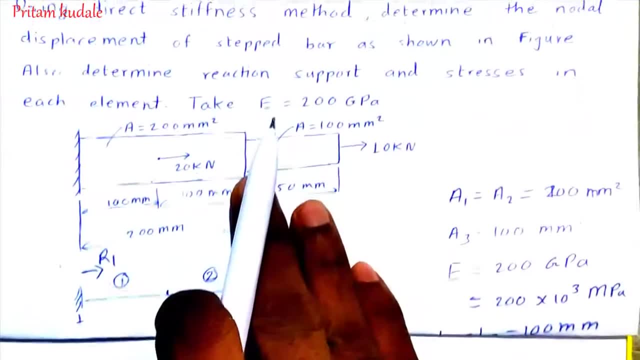 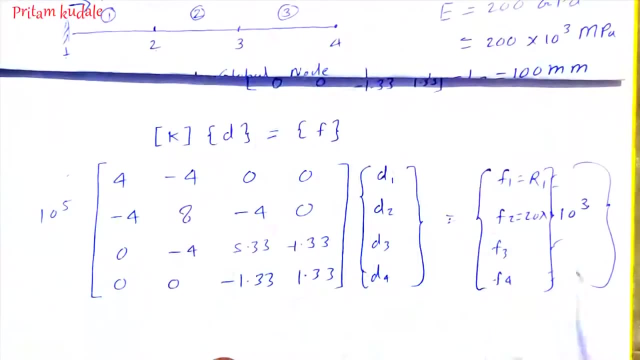 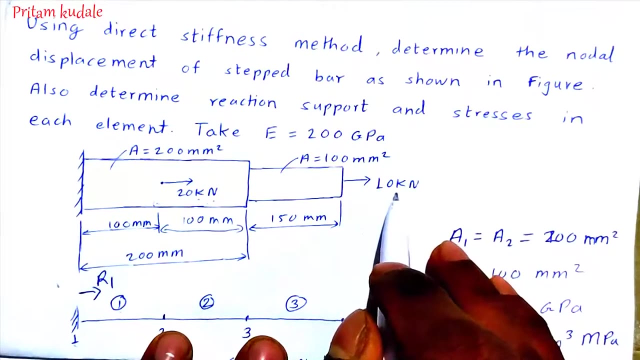 it will be 20 into 10. raise to 3. then at node 3 there is a no load available at over here, so you are going to put the value as 0. then at node 4 there is a total load of 10 kilo. 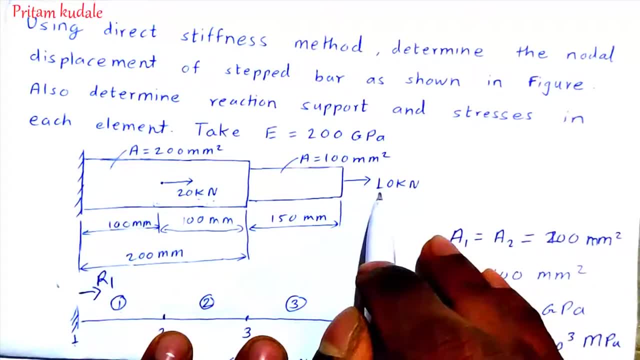 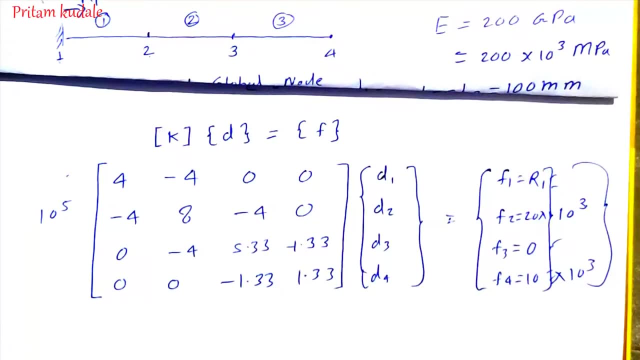 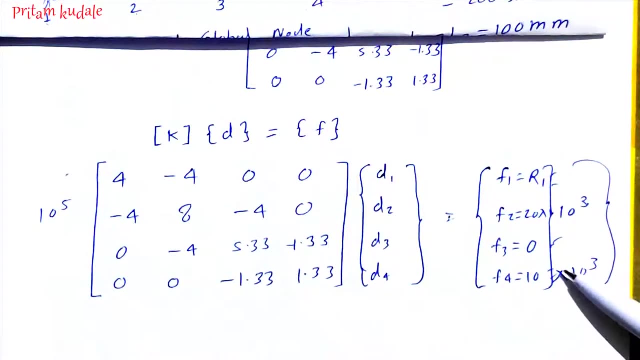 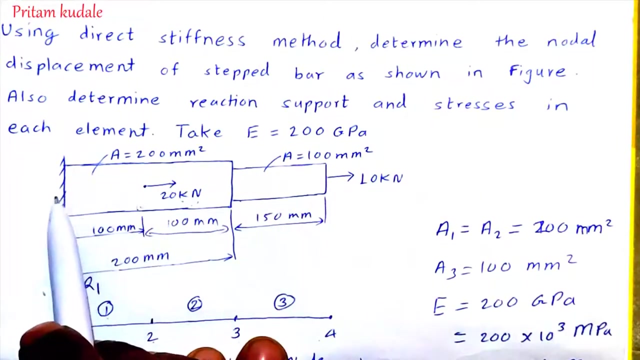 Newton. so it will be the, also in a rightward direction. so 10 into 10. raise to 3, so f4 is equal to 10 into 10. raise to 3, then this has completed our force matrix. now we are going to see a displacement now when we see here it is a peak support. so the displacement value. 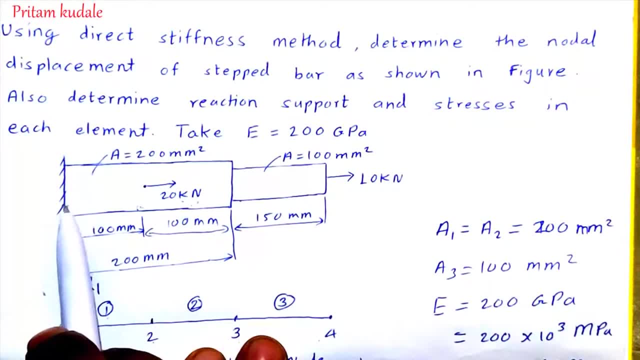 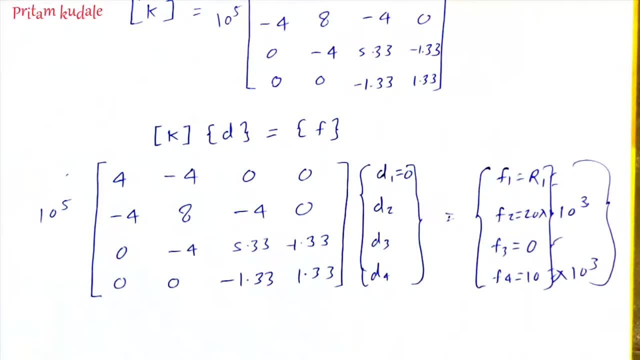 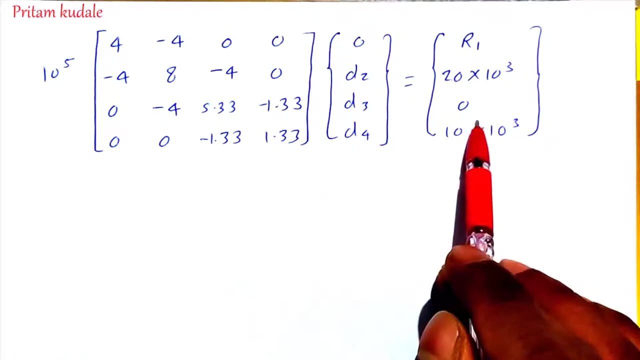 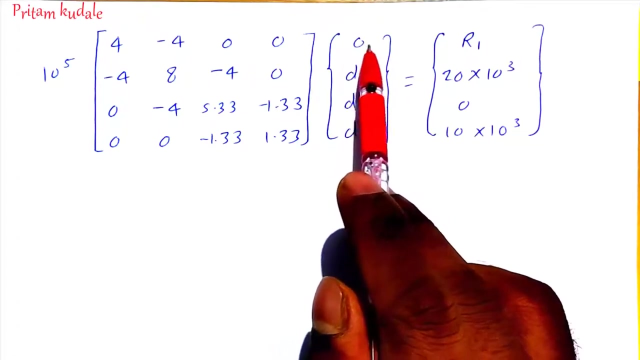 of this is 0.. that is 0 because, as it is a peak support, this particular node cannot move, so our value of d1 will be 0. ok, so this will be our final equilibrium equation. so in this equilibrium equation, wherever the peak support is given, that means there is no displacement at that. 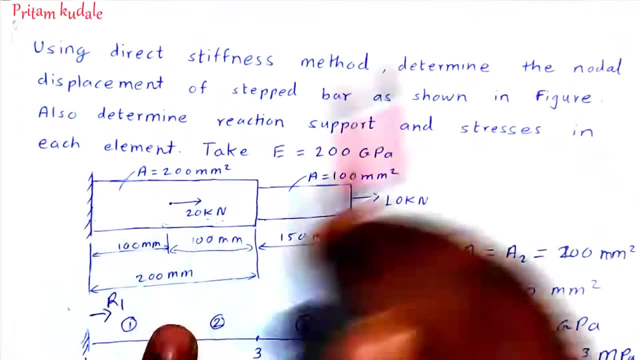 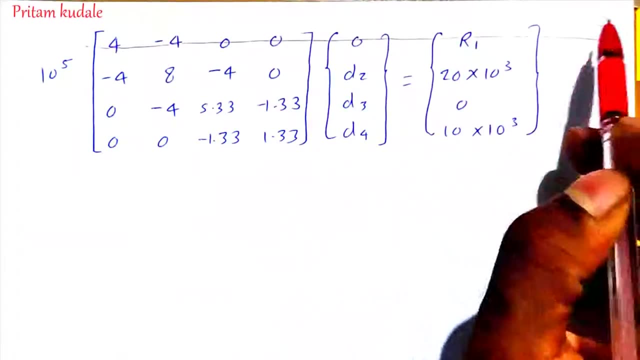 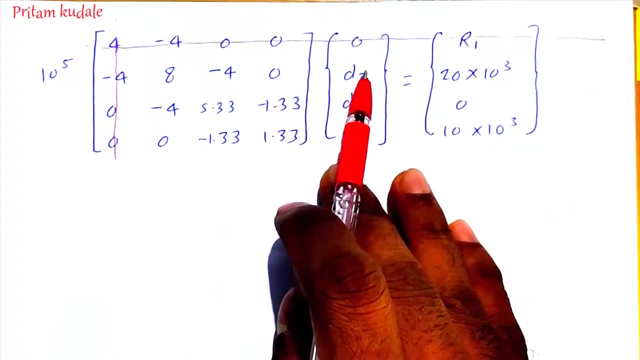 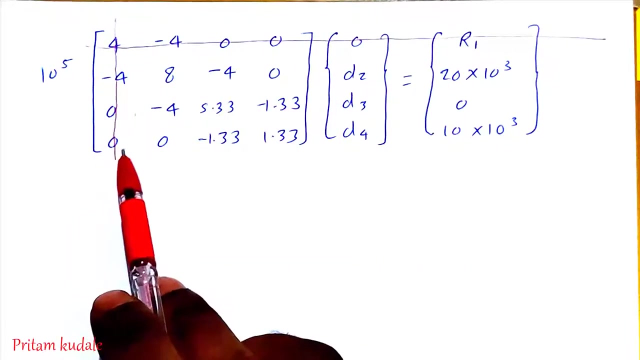 particular position we are going to. wherever the displacement is 0, we are going to eliminate that row and respective column from the global stiffness matrix. we are going to eliminate and we will rewrite this equation in a 3 by 3 matrix. that is a eliminated. whatever things are remaining, we will rewrite it now. 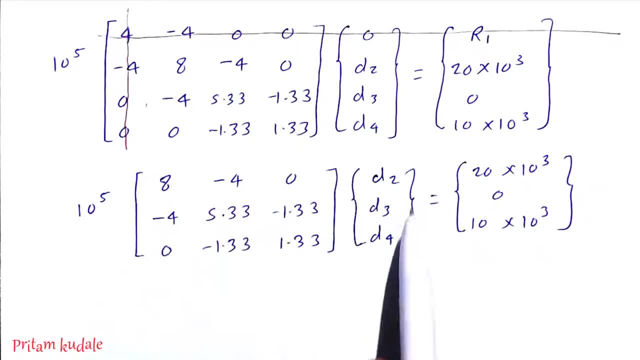 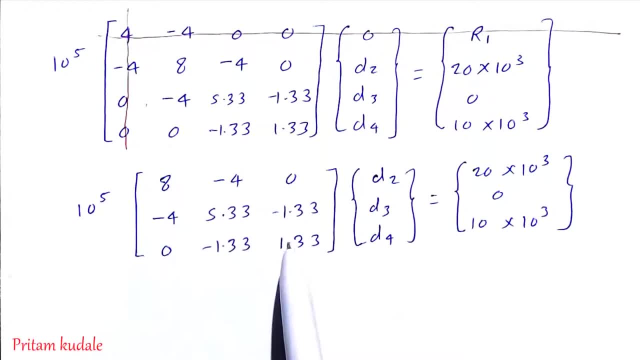 you can convert this matrix into an upper triangular form. to convert it into an upper triangular form, we have to make this, this and this value to be 0. so either you can use the RO operation or for 3 by 3 matrix, you can simple use the calculator. 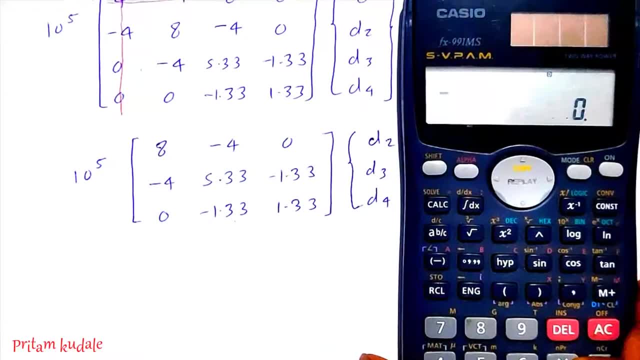 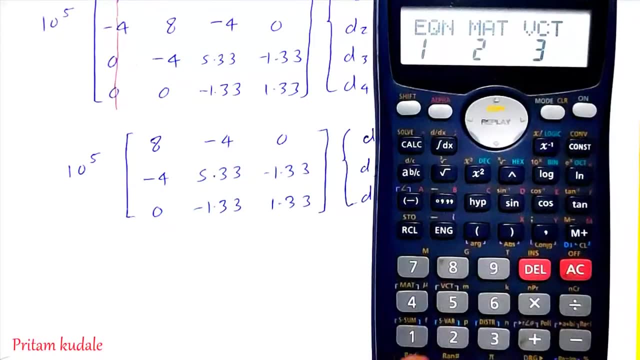 so i will show you how we are going to use the calculator to solve this problem. so, first of all, So first of all, You have to your mode into the equation mode, press the value 1 and total number of unknowns are 3. 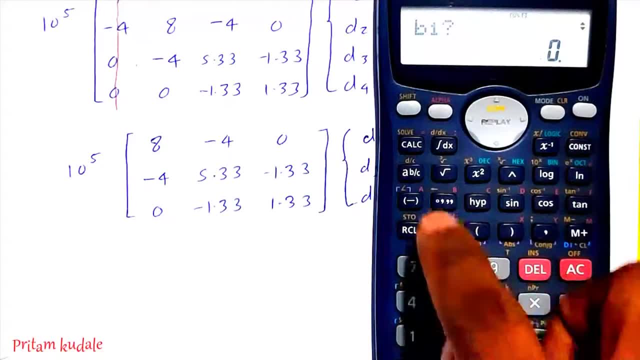 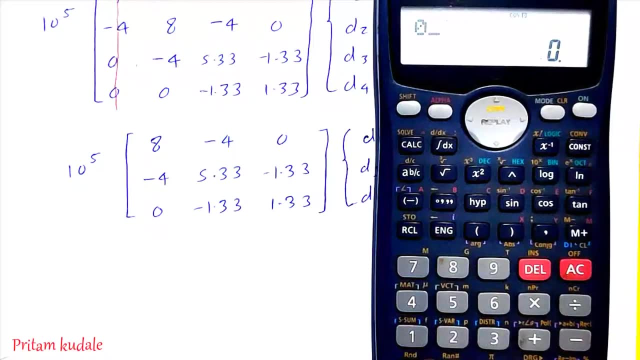 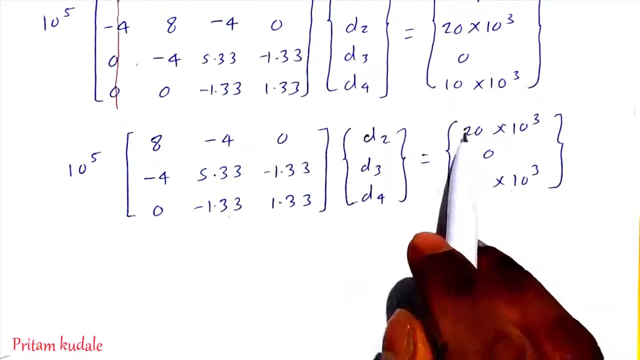 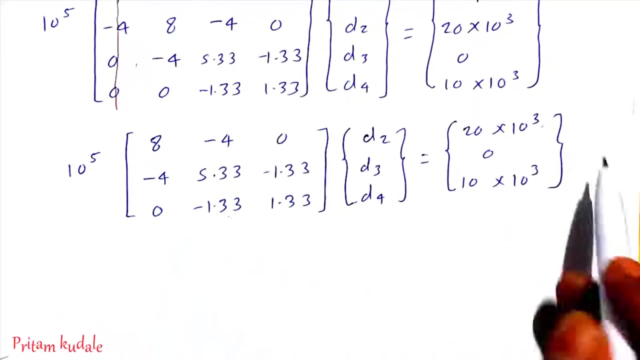 the simply, value of a1 is 8, then b1 is minus 4 and c1 is 0. and now value of d1: d1 here is 20 x 10-3, so the value of minus 10-5,. we can shift over here and it will be 0 because 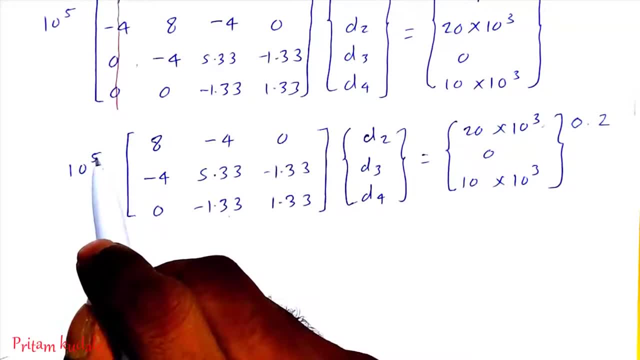 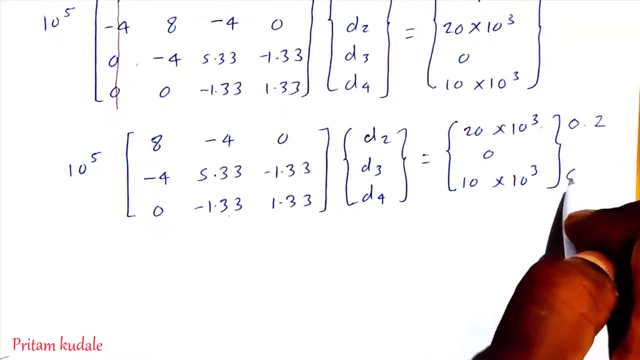 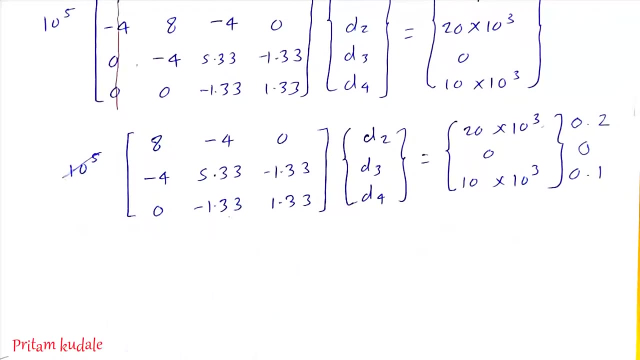 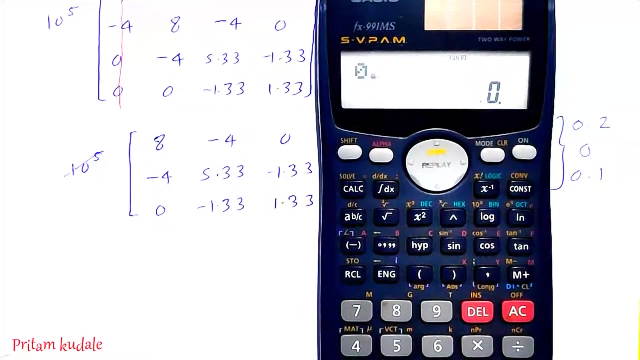 10-3 turns off, then changing the value of 10-3 will turn 20: 0 and similarly, This value is convert to 0.1 And- Surprise You- 10 raise to 5 into opposite side. So our value of D1 will be 0.2.. So we will put the value. 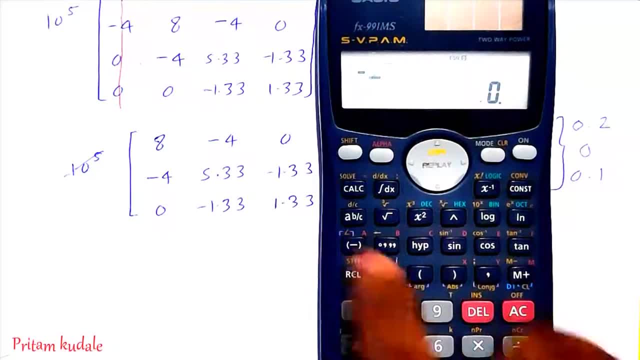 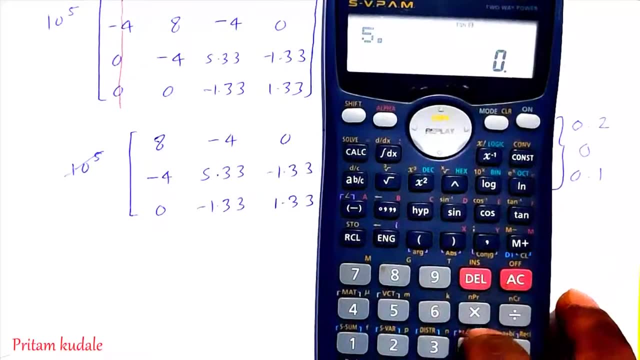 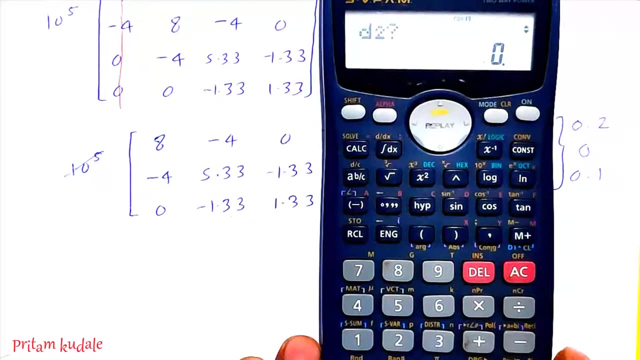 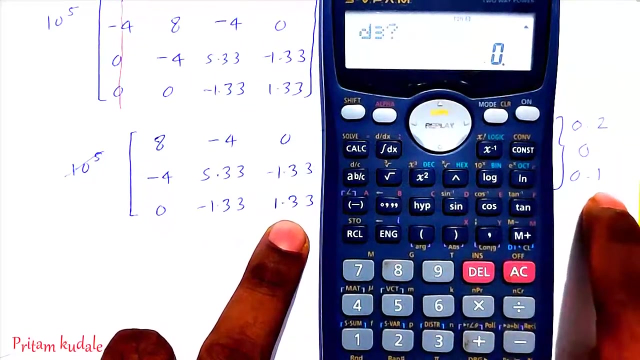 is equal to 0.2.. Now for A2: it is minus 4, then 5.33, then C2 is minus 1.33 and value of D2 is 0.. Now for third row: 0, minus 1.33, 1.33 and D1 is 0.1.. So our answers come out. 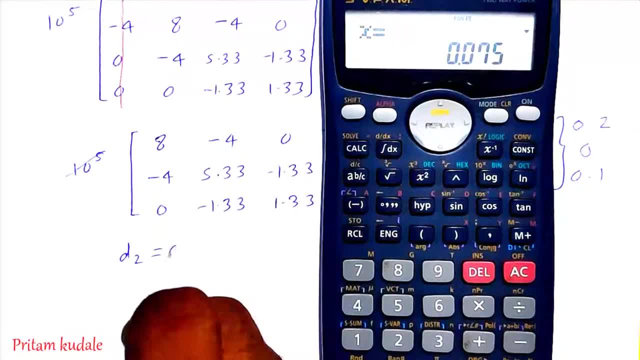 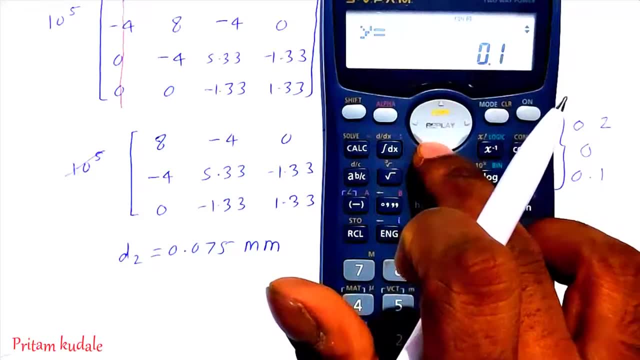 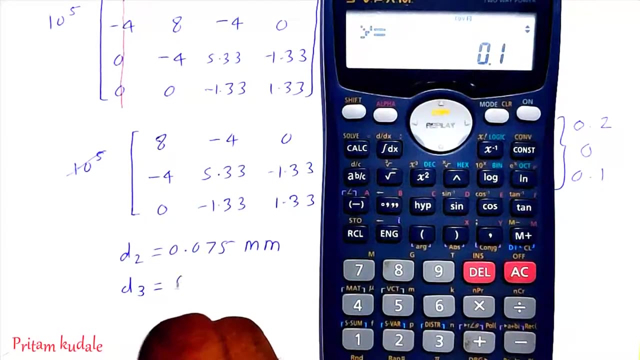 to be x. x stand for the D2, that is 0.075, and our unit will be mm. Then, second value: just put the Drop down arrow, then this will be: y will be D3.. This is nothing but 0.1 mm And value. 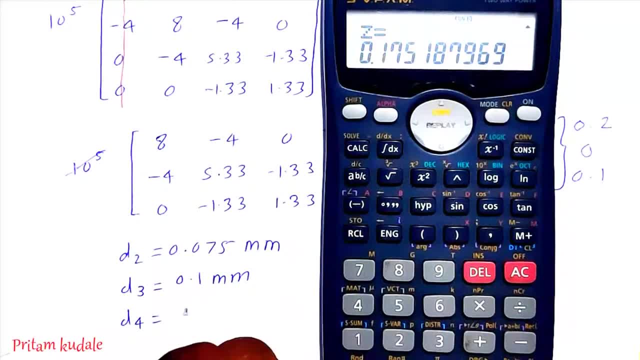 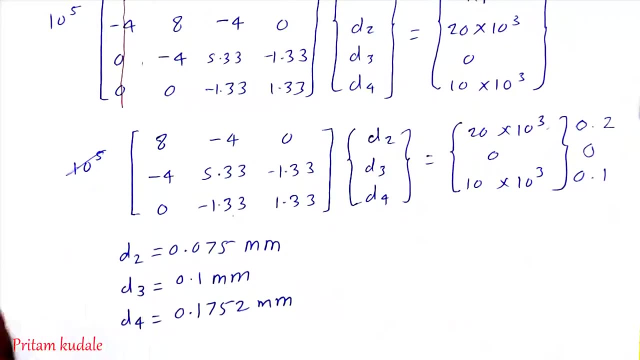 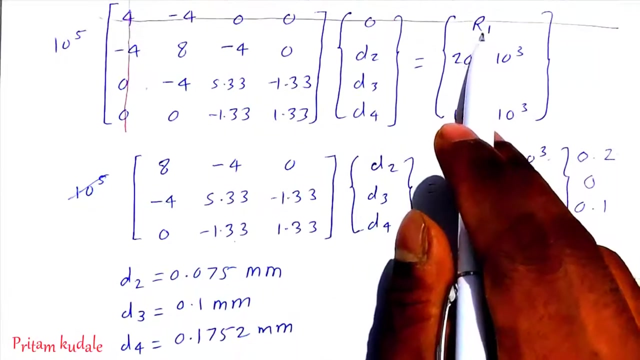 of Z stand for D4, that is, 0.175.. After 1,, 8 is coming, You can add it over here to mm. So this will be your displacement. Now, to calculate the reaction support, What we have to do? We have to go back to the upper equation. So in this equation, what? 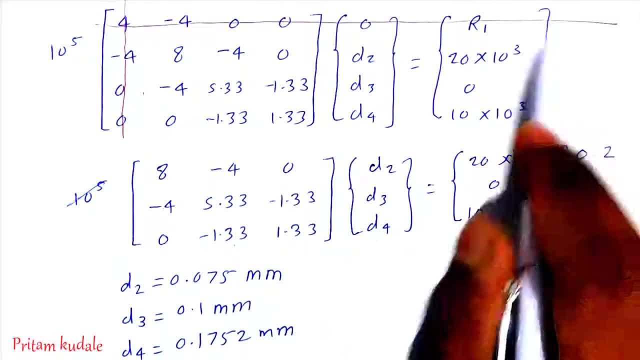 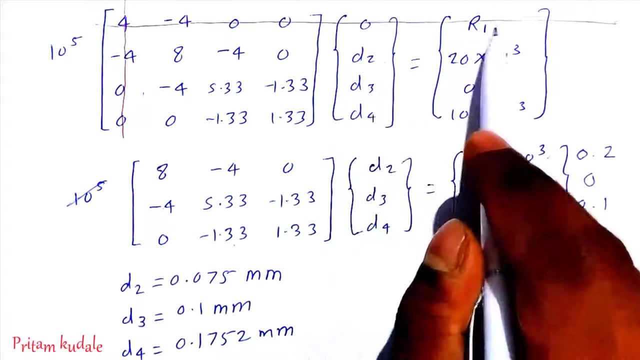 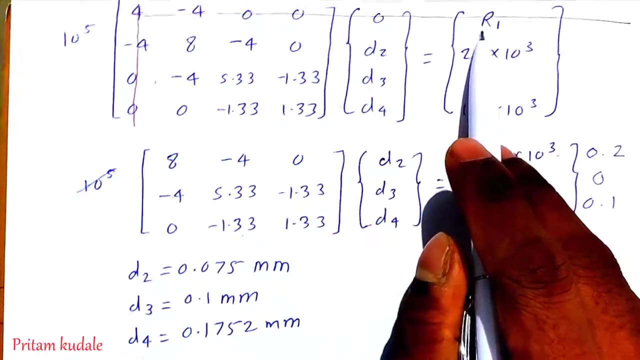 is, given that total matrices, We have to put the value of D2,, D3 and D4 and solve the equation of R1, because all are the known value. Only R1 is unknown. So first row into first column is equal to R1.. So we will write it. What is the first value is 4.. So we can write it. as a third row. Okay, Here is our equation of D4.. This is 4.. This is minus d2, minus d3.. So we can write it as a third row, Okay. So this is minus d2, minus d3, plus d1.. Now for the 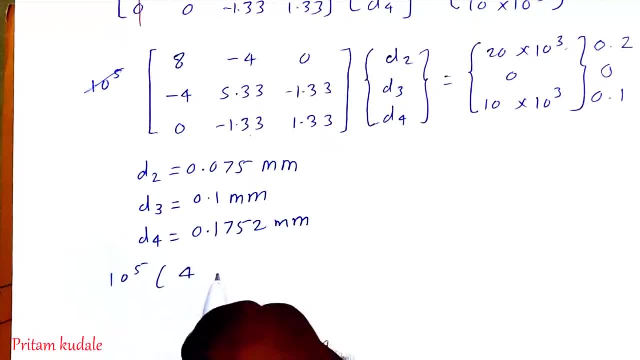 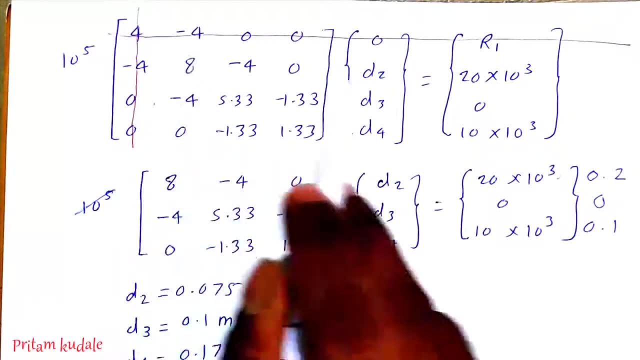 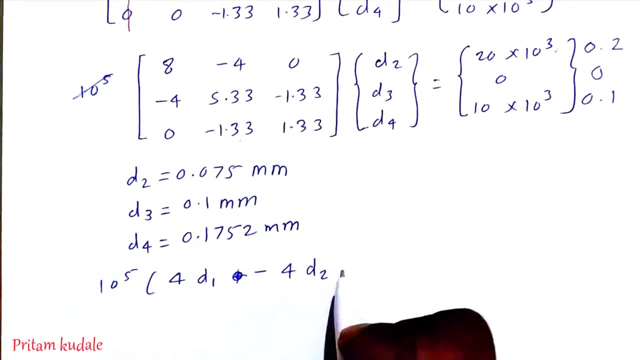 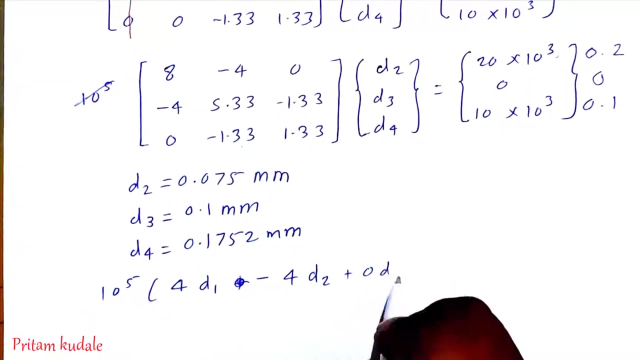 first 10 raise to 5 as it is, then 4 into d1 plus minus 4 into d2. so instead of plus there is a minus 4 into d2, then 0 into d3 plus 0 into d4, so plus 0 d3 plus. 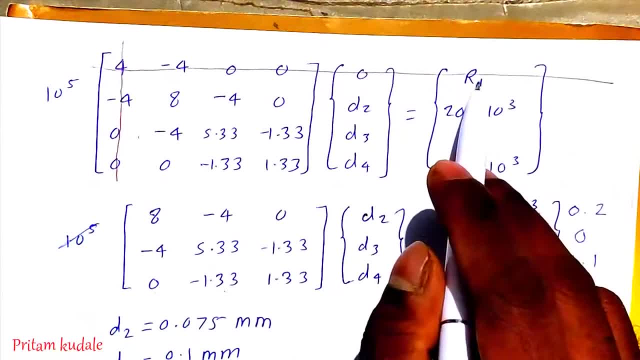 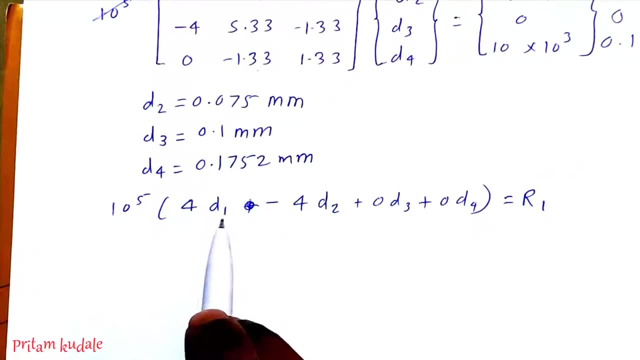 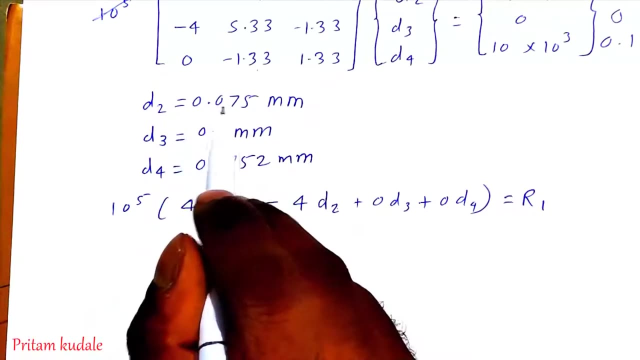 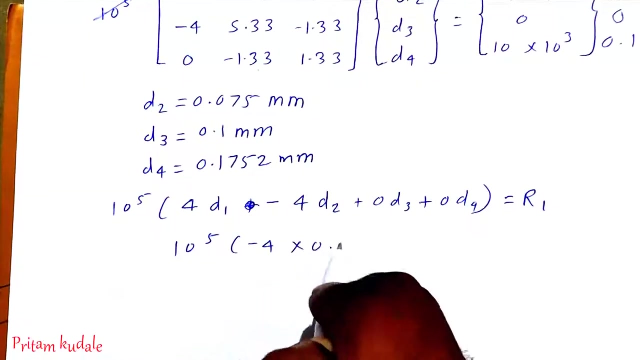 0. d4 is equal to right hand side value, that is equal to r1. so in this equation we are going to put the value of d1, which is already a 0, so this term will get cancelled. so minus 4 into d2. d2 is 0.75 mm. so 10 raise to 5 into minus 4, into 0.75, 0.075. 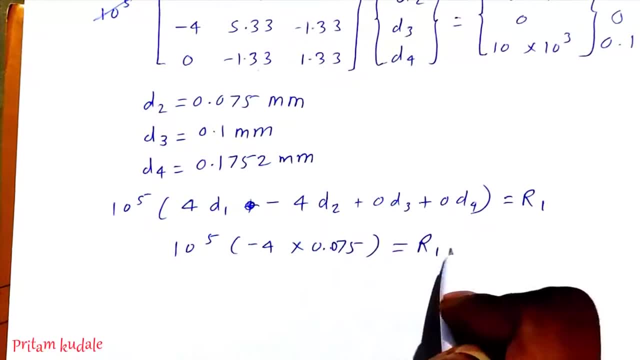 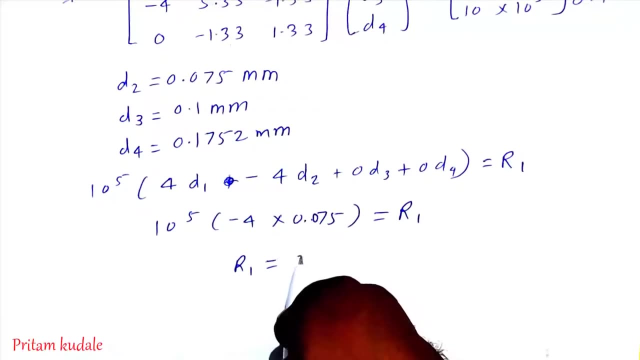 0.075. 0.075 is equal to r1, so r1 is equal to, so r1 will be equal to minus 30,000 and unit will be Newton, so which is equal to minus 30 kilonewton. so the minus sign will indicate that the our actual 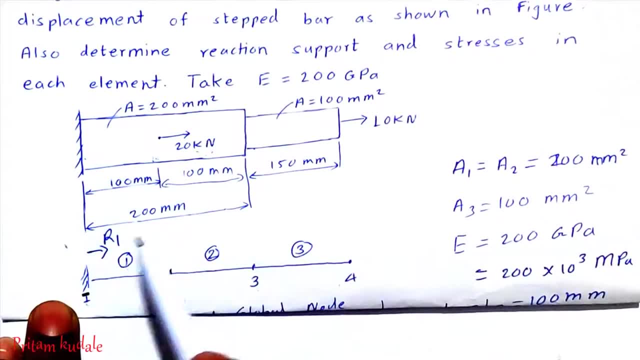 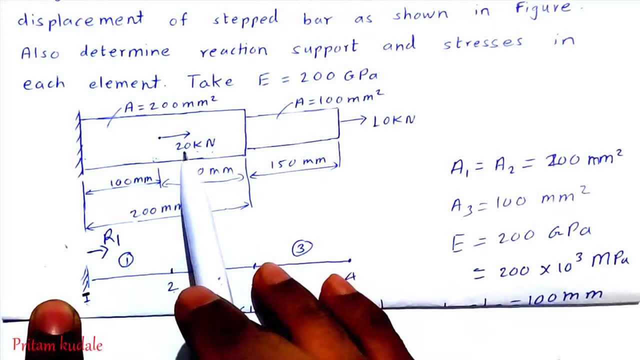 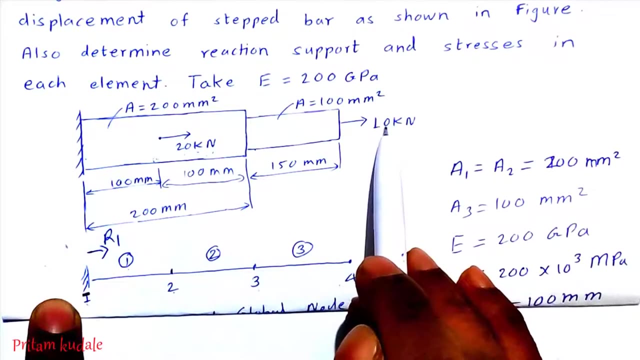 direction which we have taken, that is, in a rightward direction. so actual actual force will be in the left side direction by 30 kilonewton, and you can verify it. that is the by summation x is equal to. summation of fx is equal to 0. that is 20 plus 30, 20 plus 10, 30, though 30 kilonewton is applied in the. 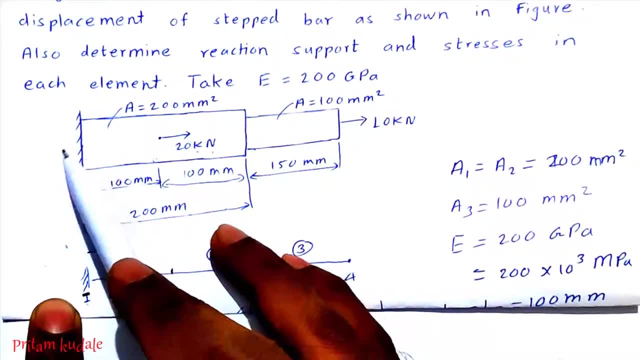 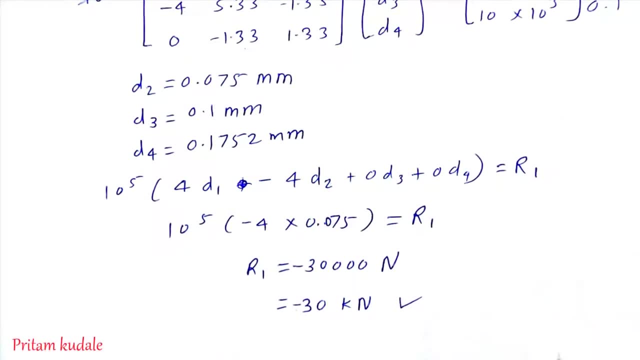 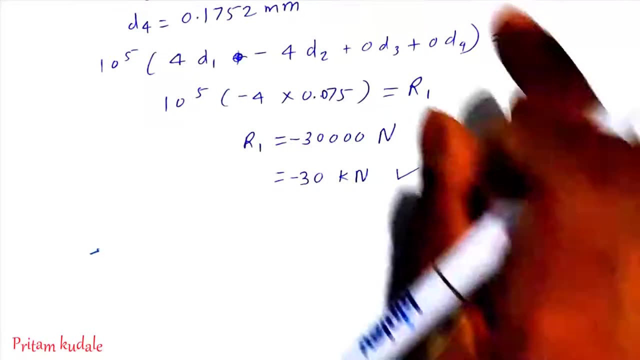 rightward direction. so definitely, reaction support will be the 30 kilonewton in the leftward direction. so our this answer is correct. okay, now we will going to see a how we are going to calculate the stress in each element. so now we totally have three elements, so there will be 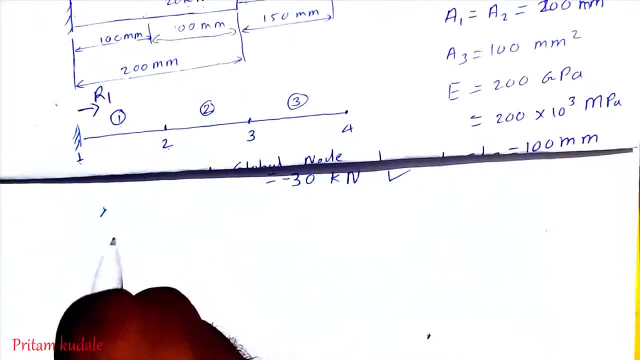 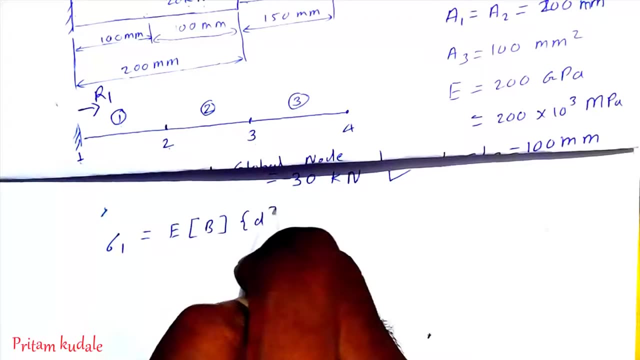 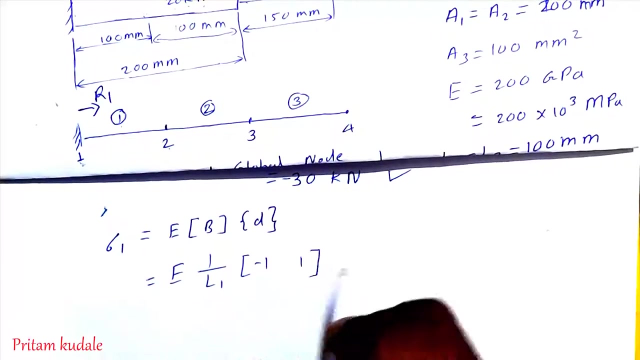 three stresses. so starting with the stress 1, that is a sigma 1, we have the formula e into b, into d. so as it is a first element having the connectivity 1 to 2, we can also write it as e is equal to b, can be write as 1 upon l1 minus 1, 1 into d having connectivity 1 to 2. so we can. 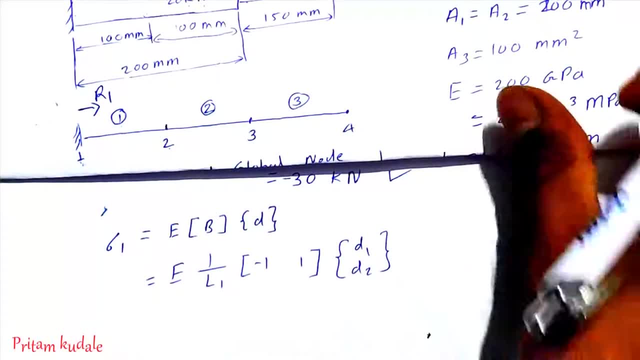 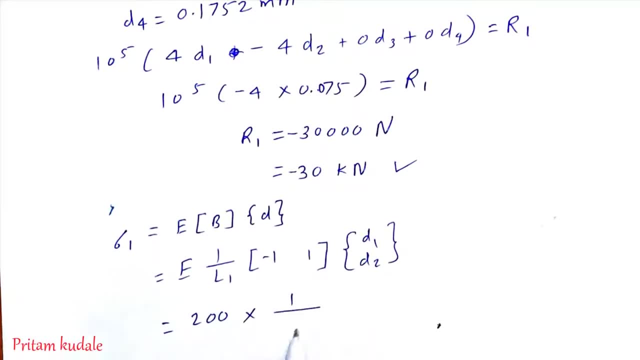 write it as a d1, d2, so we are having the all the values. that is e is equal to 200 gpa, so 200 into 1 upon l1 is equal to to 100 into 200 is GPA. so we also have to multiply by 10, raise to 3, so 1 upon 100 into. 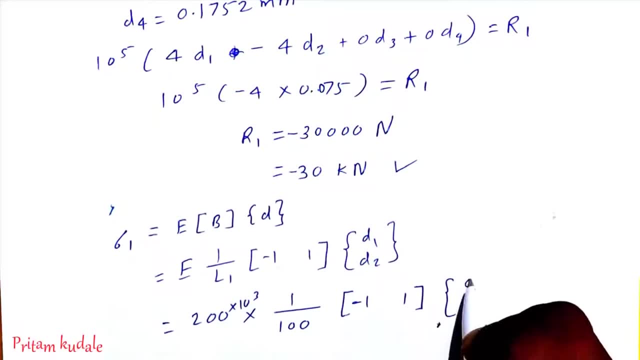 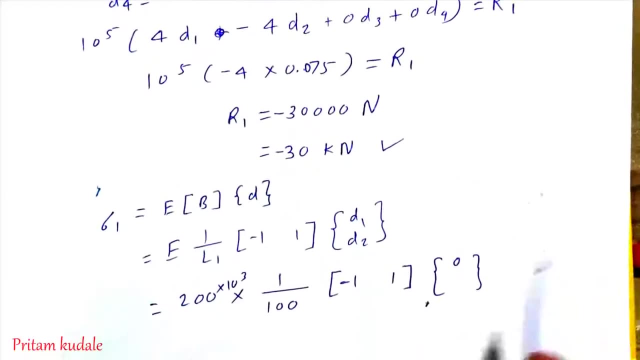 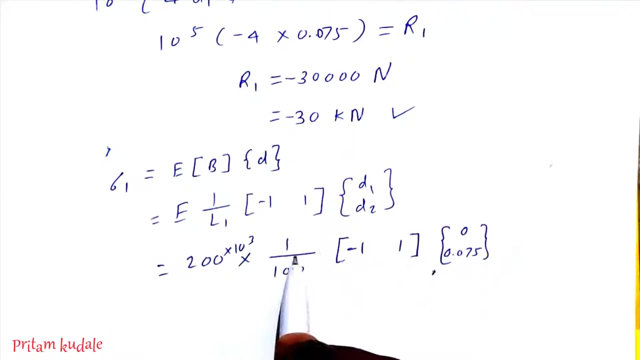 minus 1, 1 and we have already know the value of d1 is equal to 0 and d2- we have calculated that is 0.075, that we will put here 0.075. now, whatever, this is a matrix multiplication, so we have to, multiplied by first row into first column, so this will be so a 10 to 0. 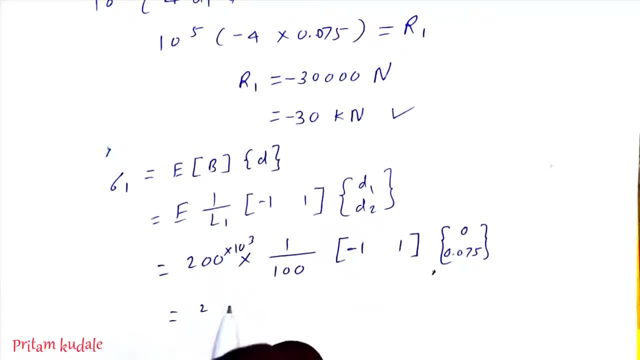 2, 0 will be cancelled. so this is 2 in 2. 10 raise to 3 multiplied by first row into first column, so 1 into 0 will be 0. so 0 Plus 1 into 0.75 is 0.75, so 0.75 into 2 So. it is very important to know that once again. so that's all for today. so a winding in this video. if you are using any common variable list, like del ii, del ii, D, vigor dvd, which are running theתanse of the reducer, so calculate thekräft feeding syntax. define both of the 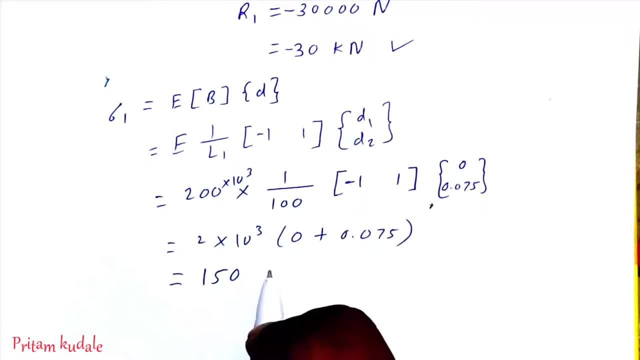 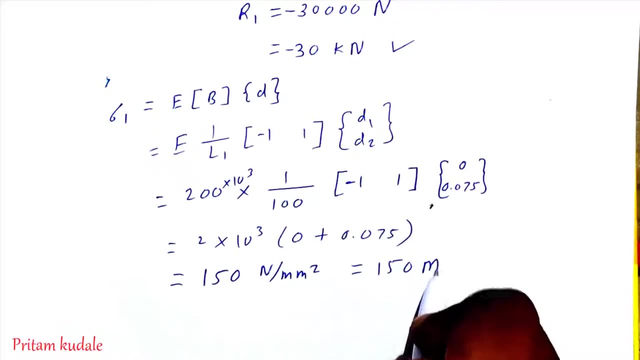 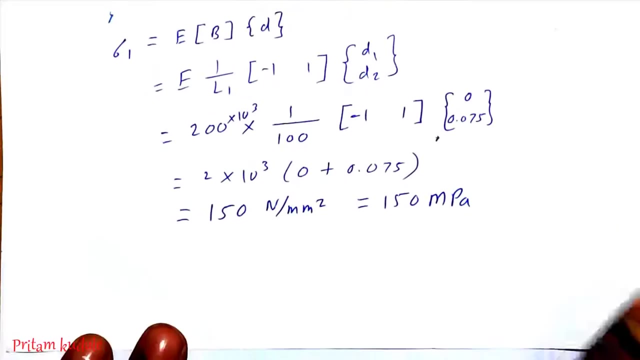 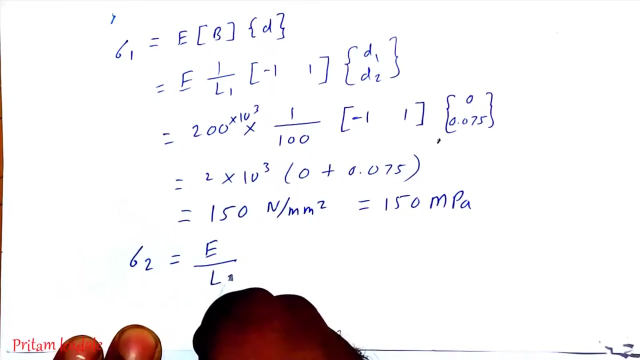 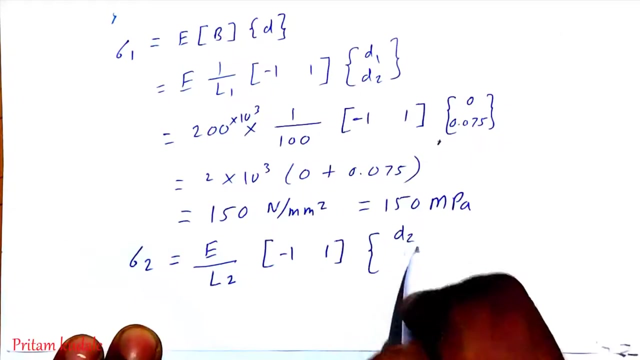 will be 150 and unit will be Newton per mm square, or we can write it as a 150 MPa. both are nothing but same. now, similarly, we can calculate: Sigma 2 is equal to now. I am going to write it directly: Sigma e by L 2 minus 1, 1, and here d 2 and d 3 as the connectivity. 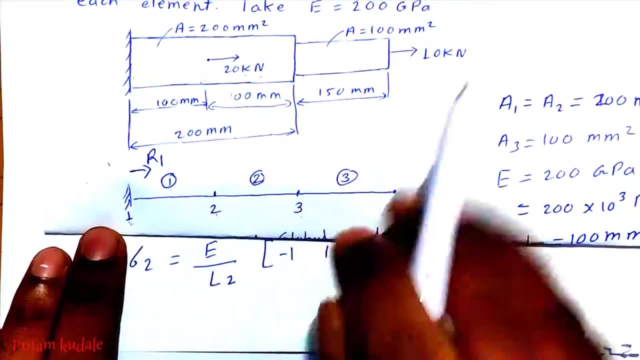 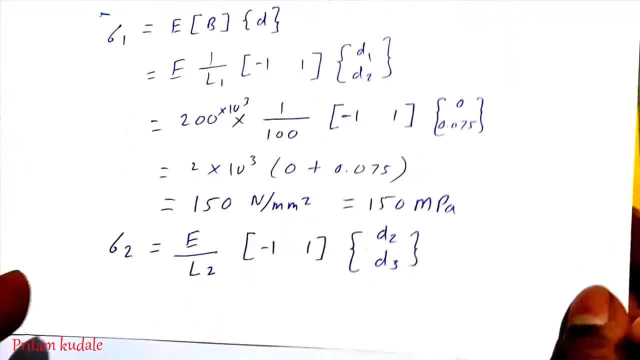 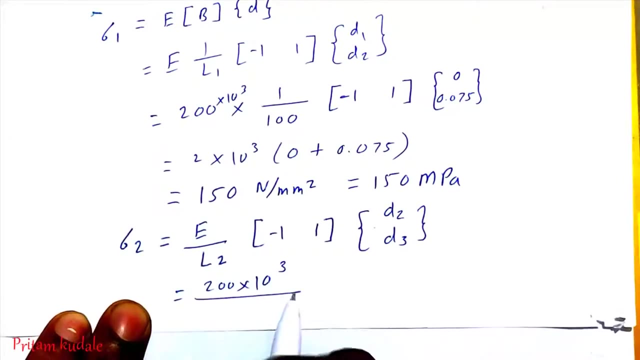 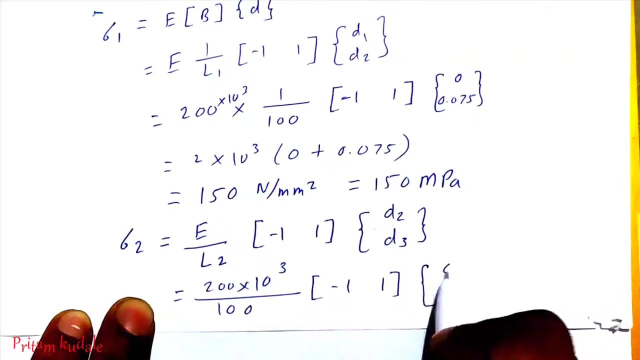 of second element is 2, 2, 3, so we already know the value of d 2 is 0.75, d 3 is 0.1, so we can put it over here. So 200 into del D divided by L 2 is nothing but 100 minus 11 and in column 0.05 and 0.1. so 1 into minus. 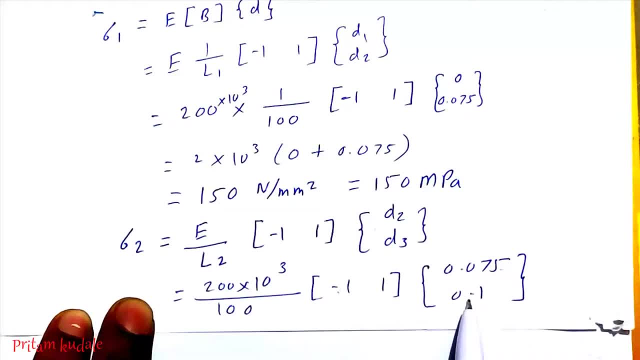 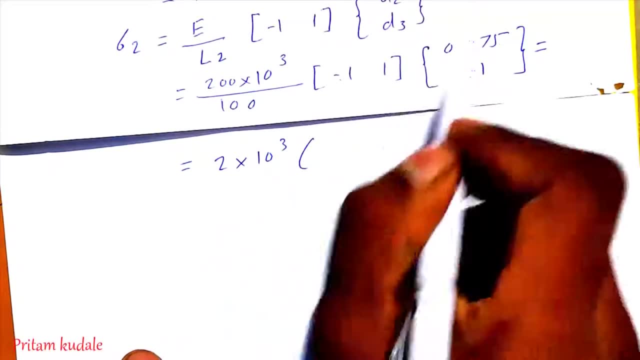 1 into 0.75 plus 1 into 0.1, so this is 2 into n, result 3 into bracket. 1 into minus 0.7, so minus 0.07, as the connectivity of second element is very simple.